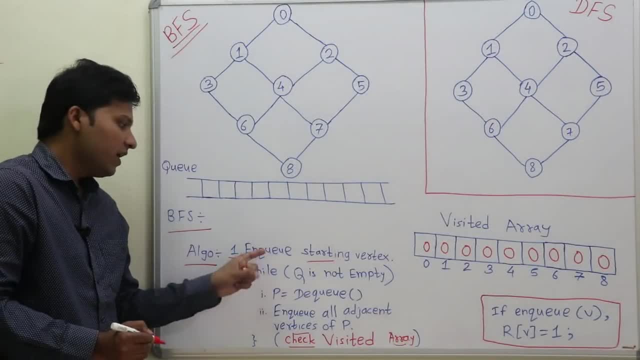 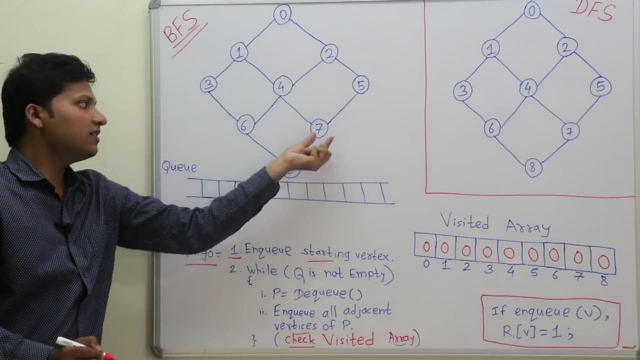 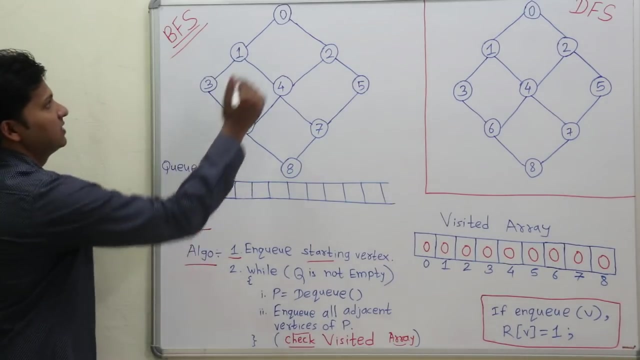 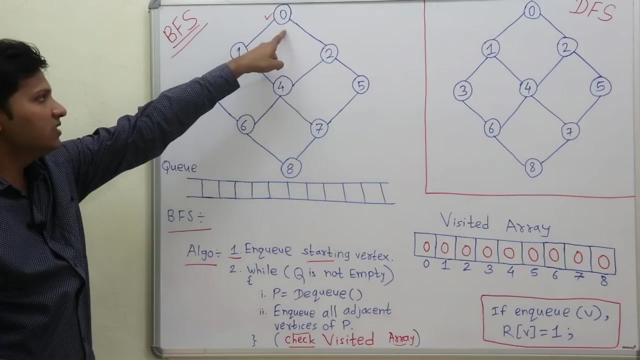 algorithm. Now, the first step in the algorithm is NQ starting vertex. So the starting vertex is the vertex from where you want to start printing the BFS traversal. So you have to decide the starting vertex. Now we will decide. the starting vertex will be 0.. Now, after you decide the 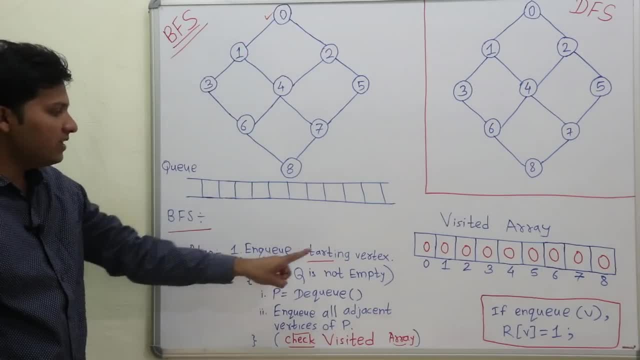 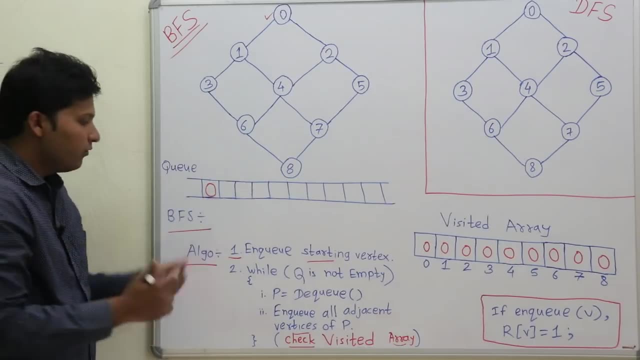 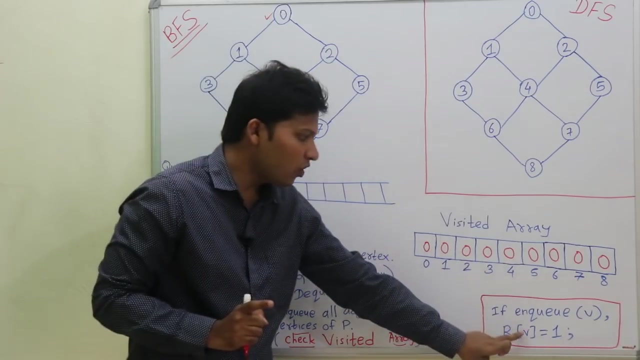 starting vertex, you have to NQ that starting vertex. Now I NQ the starting vertex here. So there is a rule for every NQ operation. So whenever you NQ a vertex, you have to follow this rule. This is one rule. So if you NQ vertex, 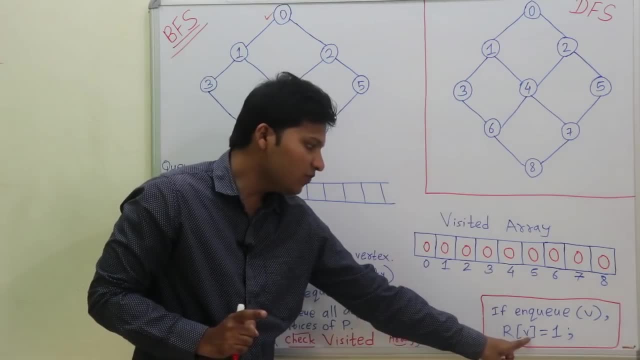 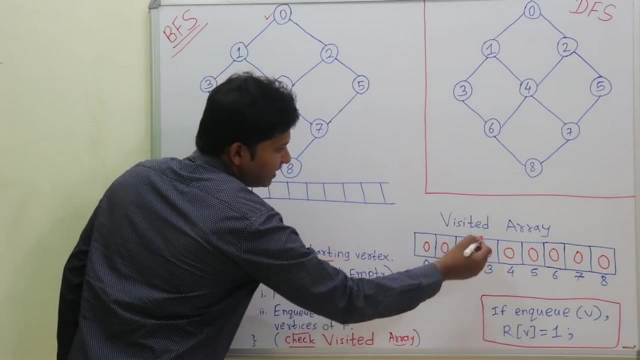 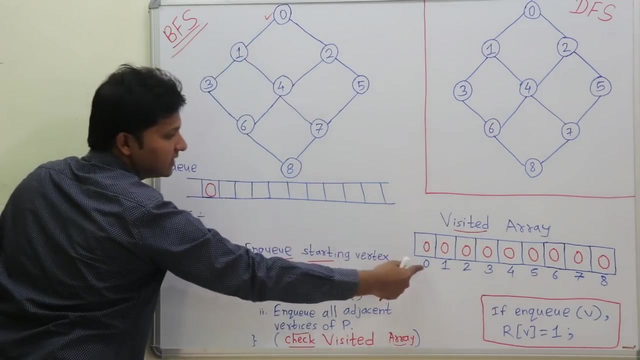 V you have to set the value of that vertex is equal to 1 in this array. So this is the array and this array is called as the visited array. So for vertex 0, as this vertex is now visited because it is NQ'd. 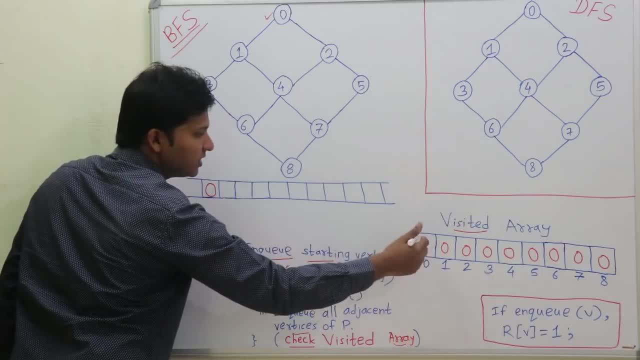 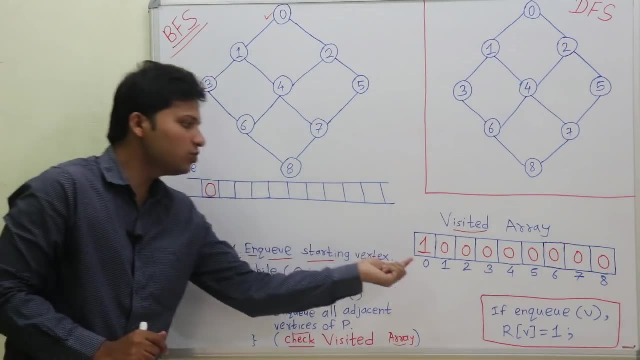 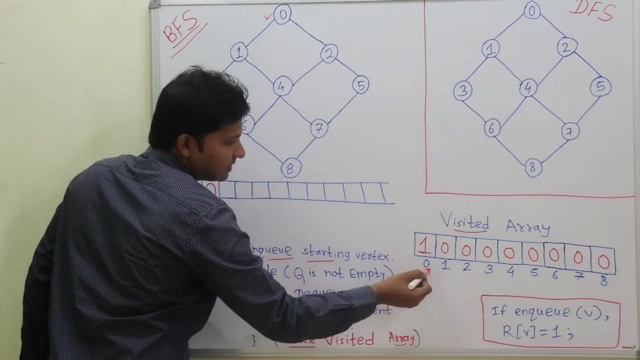 In the queue you have to set the value is equal to 1.. This is simple, See: whenever you NQ a node in the queue, you have to set the value as 1.. Okay Now. so for this array, the index is 0,, 1,, 2,, 3,. 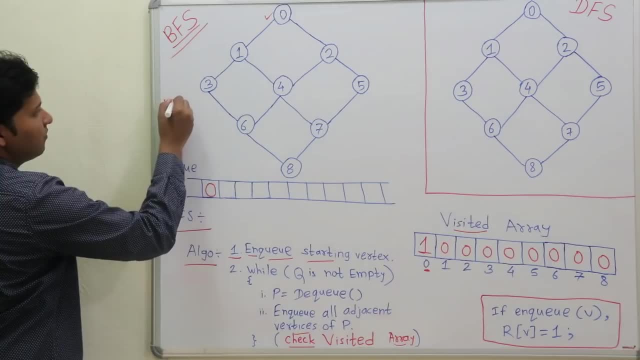 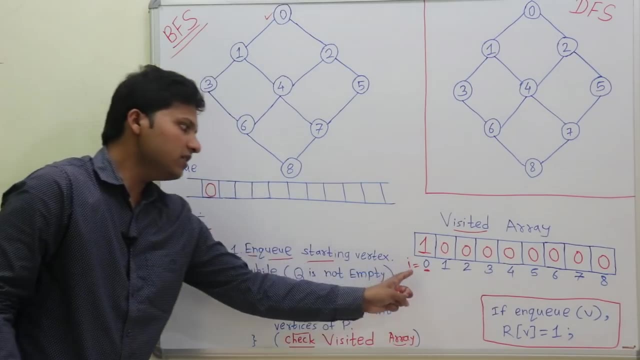 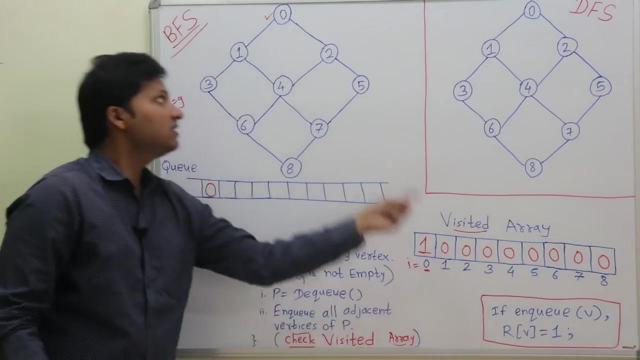 4 up to 8, because there are 9 vertices in this graph. Okay, So the index i is denoting the vertex. Okay Means the index 0 is the vertex 0.. The index 1 is the vertex 1.. The index 2 is the. 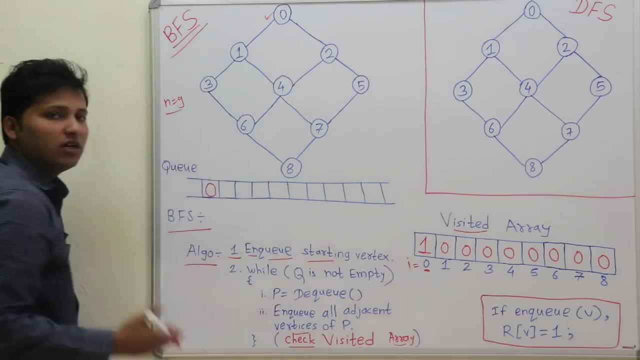 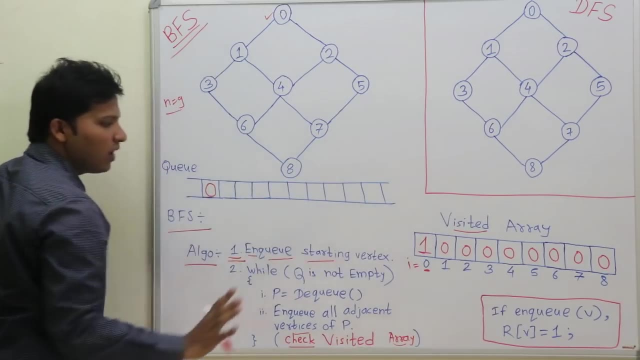 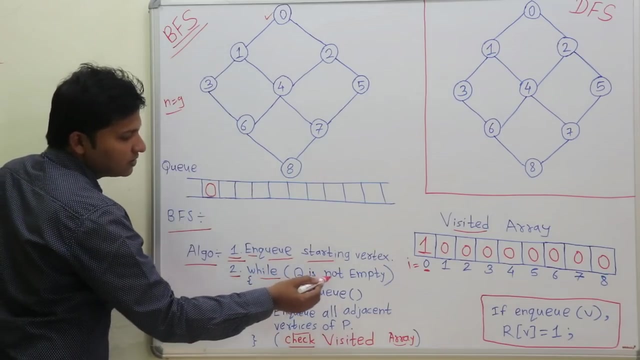 vertex 2.. Okay, So the index is equal to the vertex. So the first step is over. You have NQ'd the vertex and you have set the value as 1.. Now let's go to the second step. The second step is while queue is. 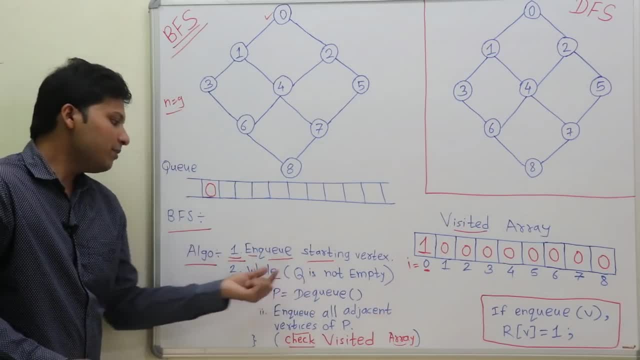 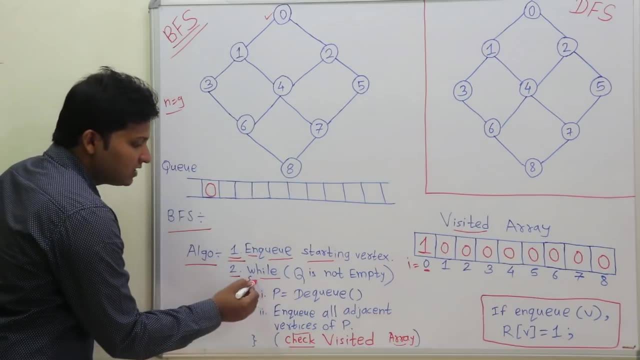 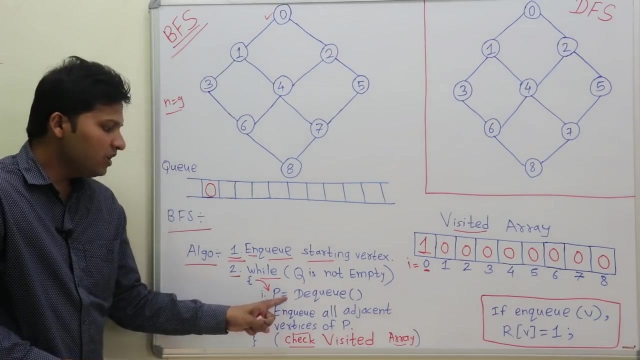 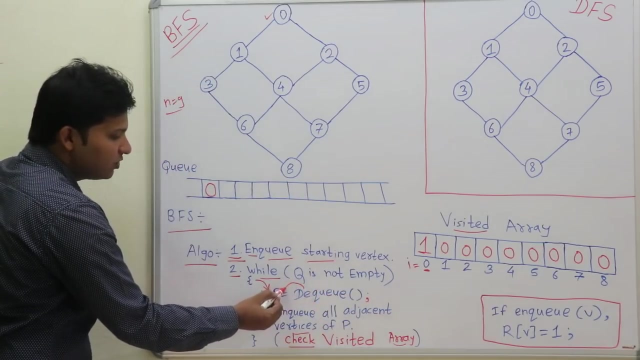 not empty. So while queue is not empty- condition is true here, because there is one vertex in the queue- The queue is not empty. So let's go inside this while block. Now the first step inside this while block is: p is equal to dq. Okay, So if you want to dq the node, you have to assign the dq node to the pointer p, So p. 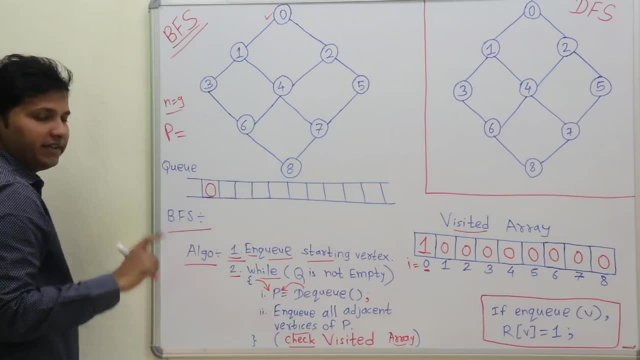 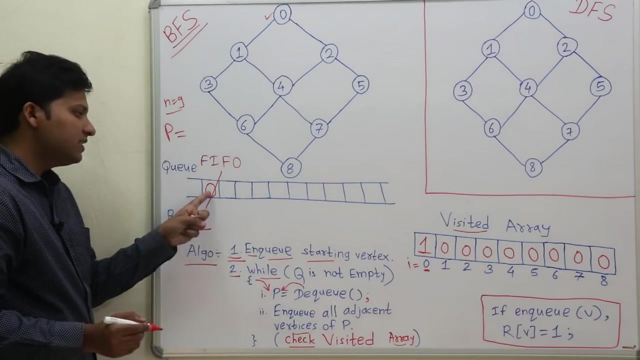 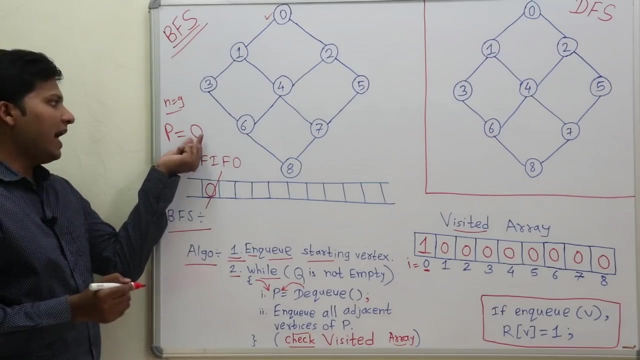 is a pointer or it is a variable pointing to the dq'd vertex. So now the dq'ing vertex is vertex 0, because inside the queue, as queue follows first in first out procedure, now the vertex 0 will be dq'd. So now p points to vertex 0. So p holds the. 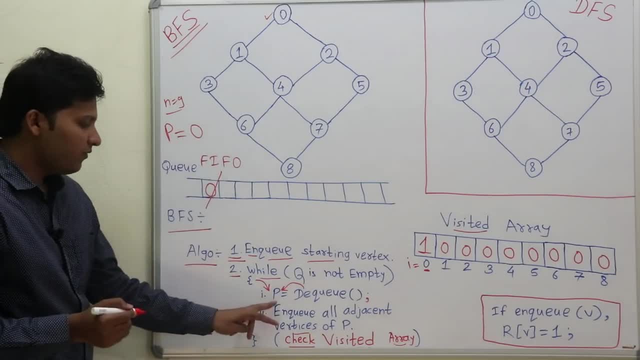 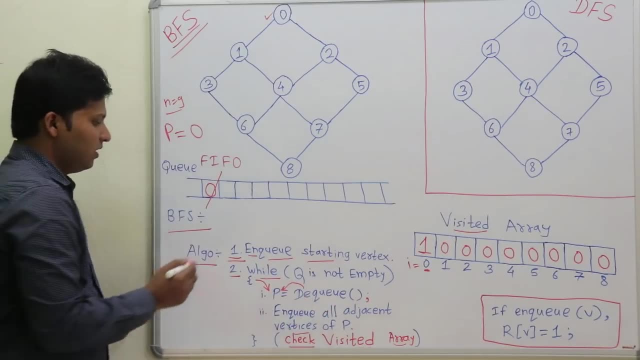 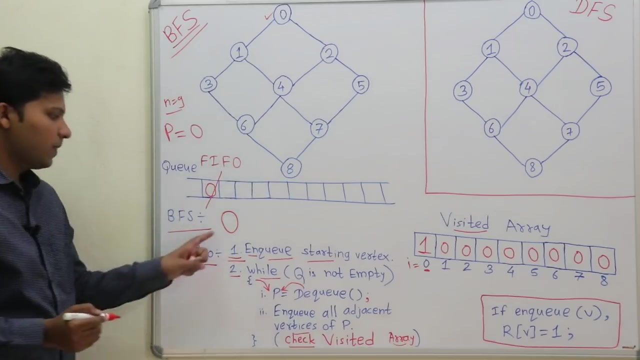 address for vertex 0 now. So after you do this step, you have to print the value of that dq'd node as the bfs traversal. So the node dq'd is 0. So print 0 now. okay, So for every dq' operation. 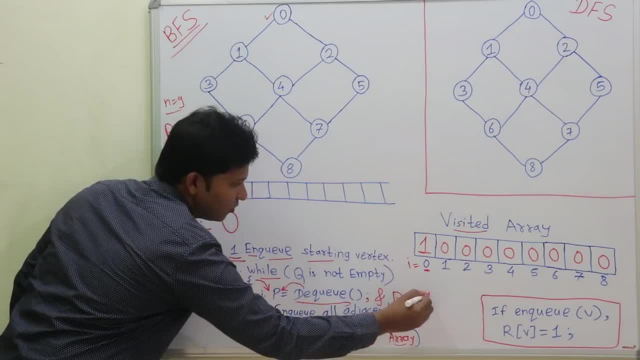 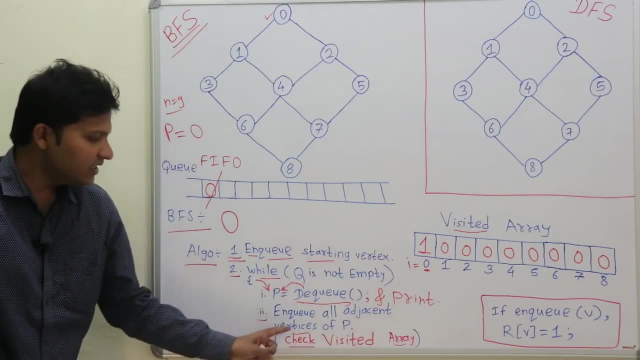 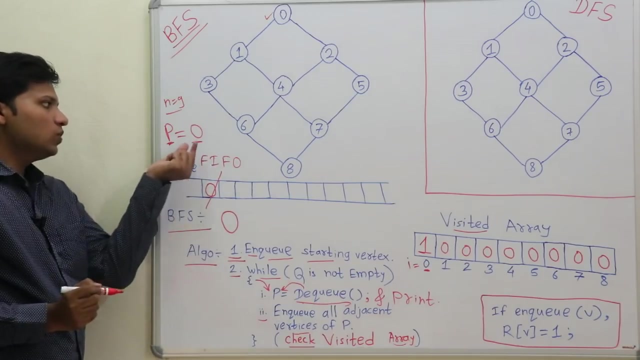 you have to dq and print that node. okay. So now the second step. see nq, all adjacent vertices of the vertex. P means the vertex pointed by p. So now the vertex is 0.. Now p points to vertex 0. So we find the vertex in dash at dv. We have dv'n plus 0. Now p can follow. 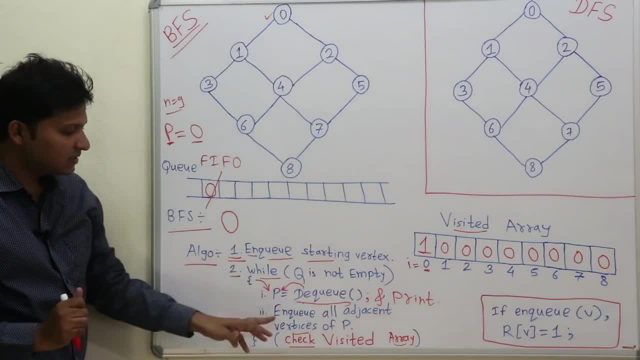 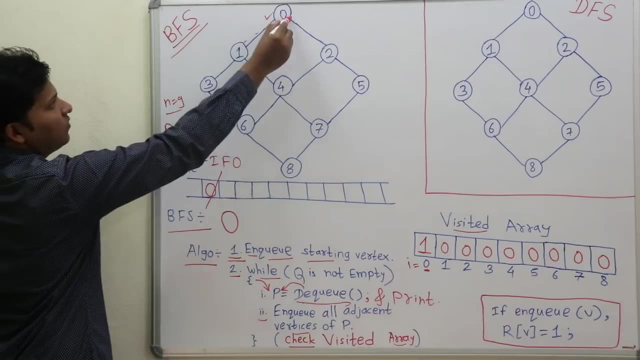 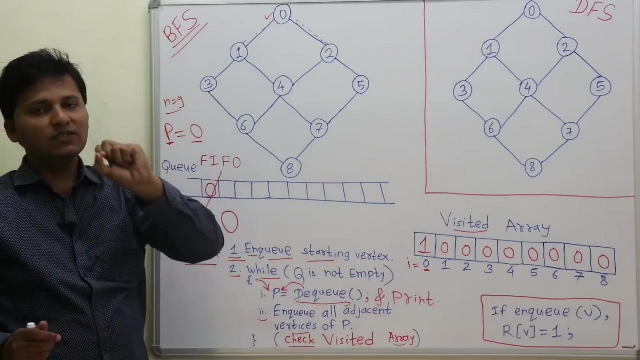 projections depending on the dq'심. After dq you have to and produce a group so that the vertex is is 0.. So what are the adjacent vertices of vertex 0? here? See, the adjacent vertices are vertex 1 and vertex 2.. Now the question is that what is a adjacent vertex? So the vertices which share. 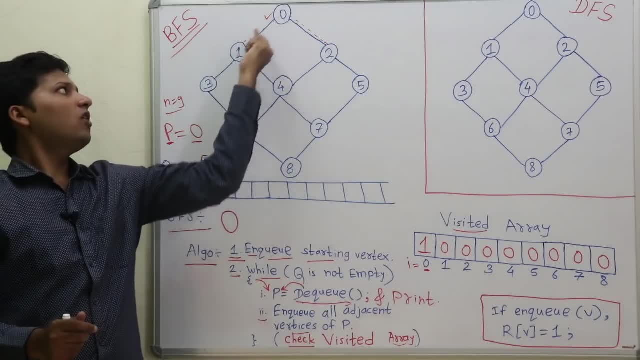 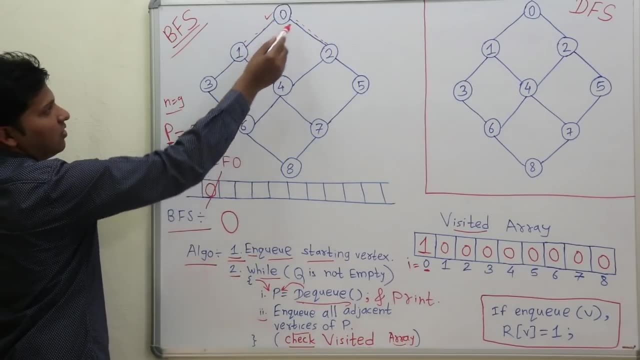 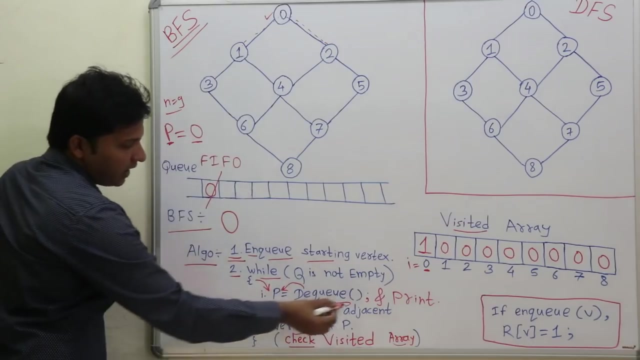 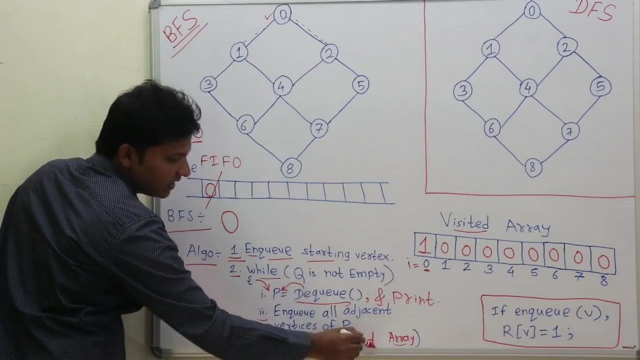 an edge between them are called as the adjacent vertices. See here: vertex 0 and vertex 1 share an edge. Vertex 0 and vertex 2 share an edge. So they are adjacent vertices. So now enqueue all the adjacent vertices. But before enqueuing you have to check the visited array first. I will tell. 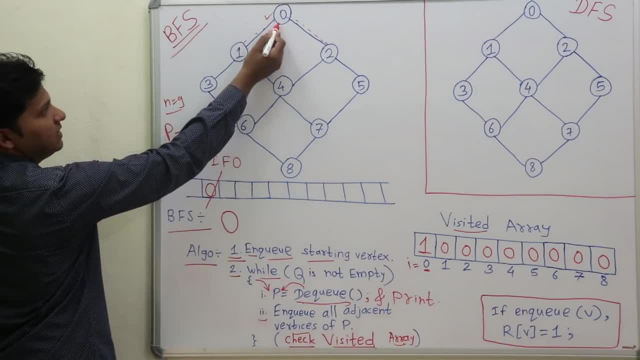 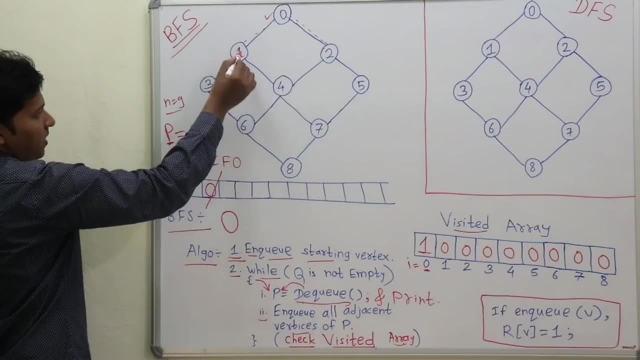 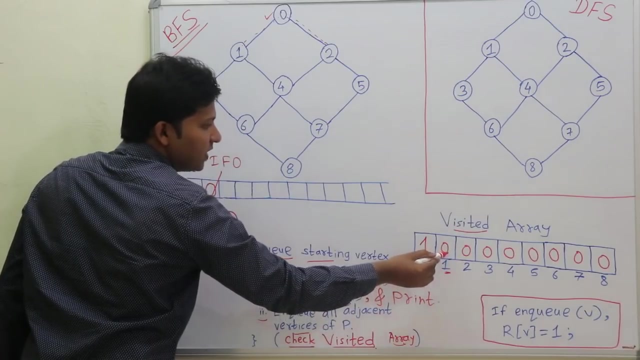 you what's the meaning of this? See for vertex 0, the adjacent vertex is 1 and 2.. So let's start with the first vertex, that is 1.. So you have to check the visited array for vertex 1.. So the value at vertex 1 is 0 means this vertex is yet unvisited. 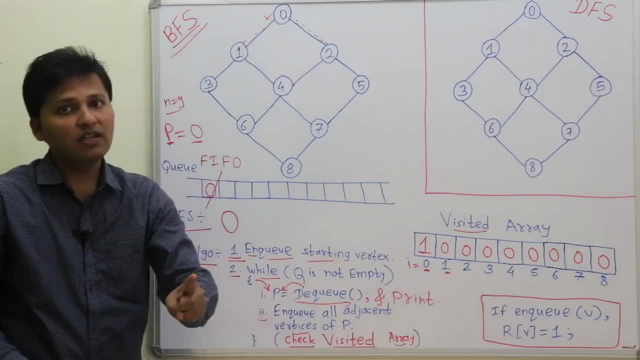 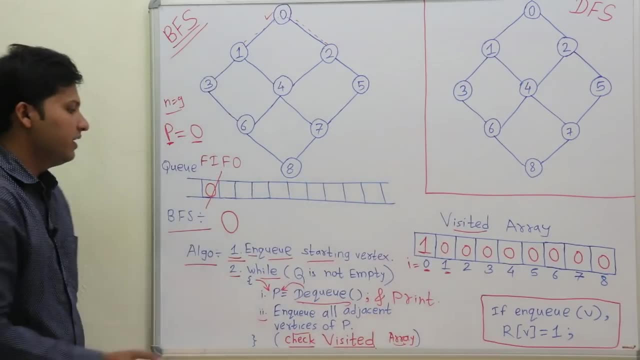 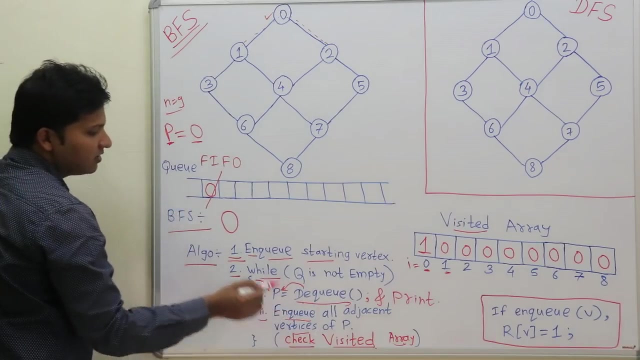 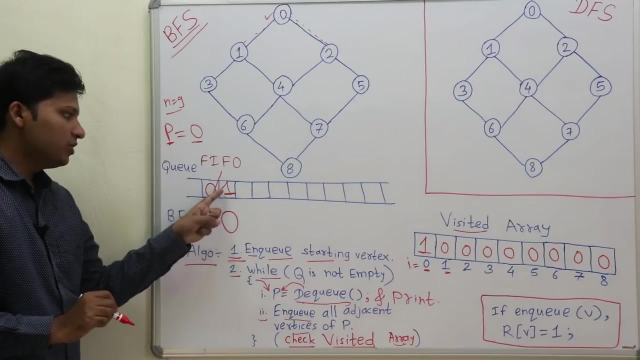 and if it is unvisited, then only you can enter that vertex in the queue, Then only you can enqueue that vertex. So at vertex 1 the value is 0 means it is unvisited, So you can enqueue that vertex. So let us enqueue 1.. So now, vertex 1 is enqueued, means it is now visited. So when it is visited, 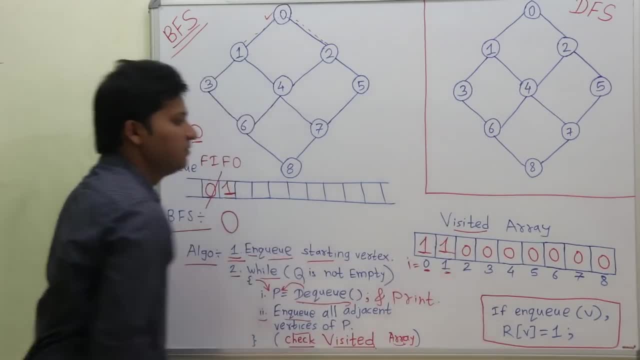 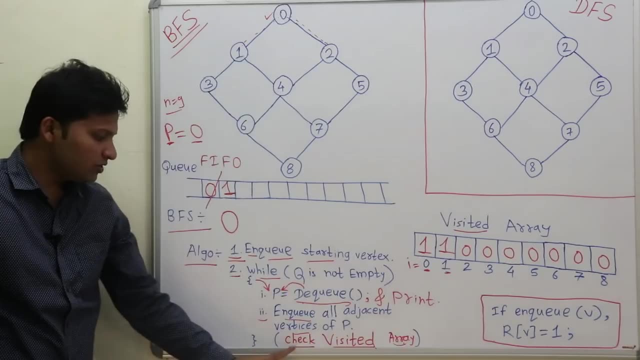 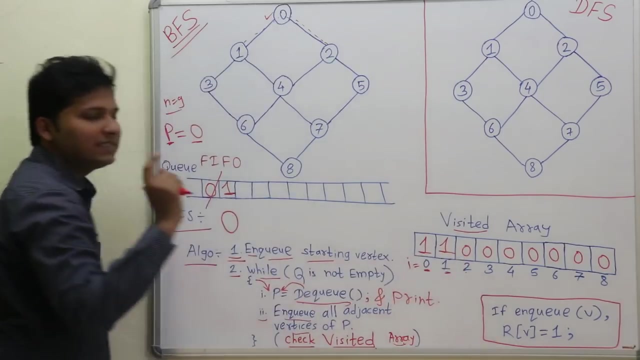 you have to set the value as 1.. Now let us go to the second vertex, the vertex 2.. So now for vertex 2. also, you have to check the visited array. Now for vertex 2. yes, the value is 0 means that. 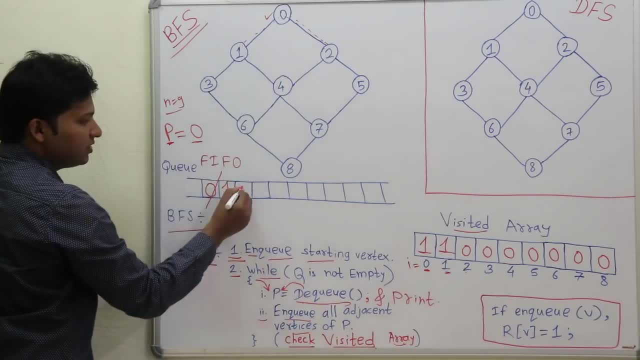 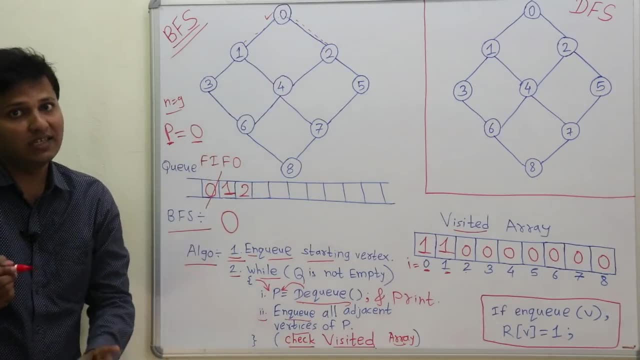 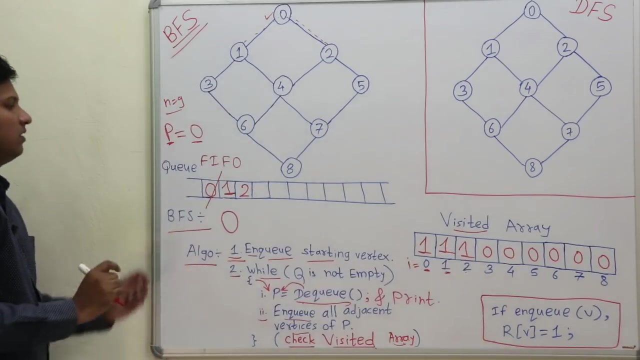 vertex is yet unvisited, So you can enqueue that vertex. and when you enqueue that vertex, that means this vertex is now visited. So, as it is visited, you can set the value as 1 here. Now see, these two steps are over. 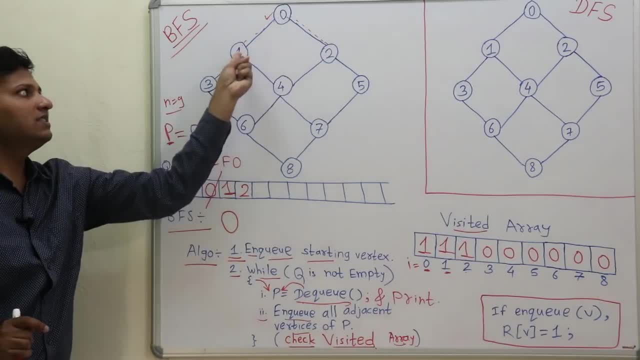 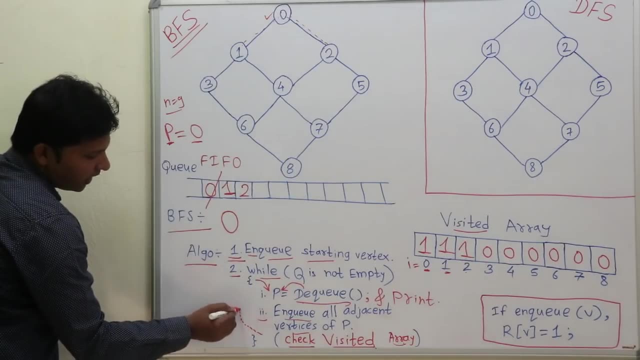 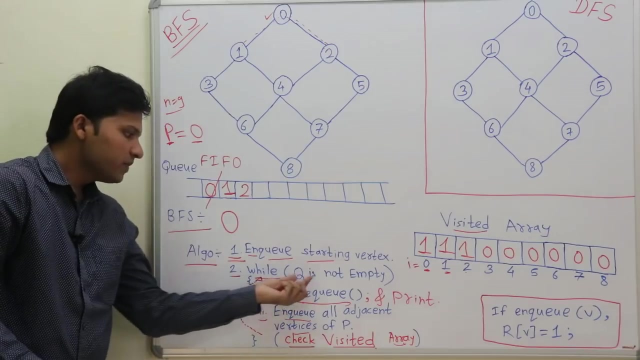 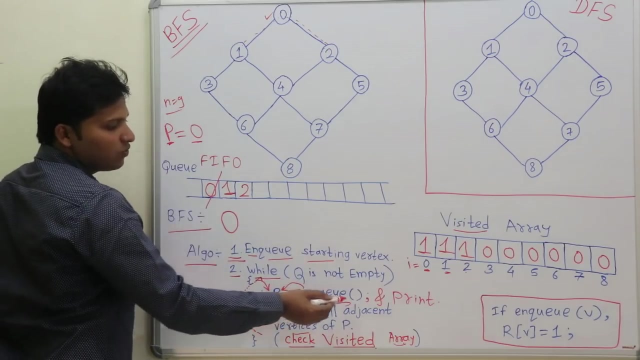 because all the adjacent vertices for vertex 0 are entered inside this queue. Now, as this is visited, you have to iterate to the next while loop. So let us go to the next while loop. Yet the queue is not empty, So let us go inside and follow the first step. So the first step is: p is equal. 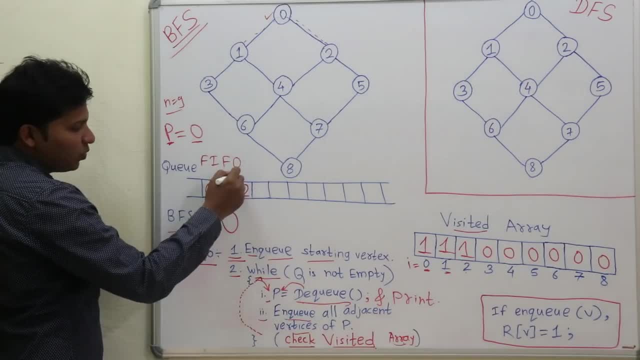 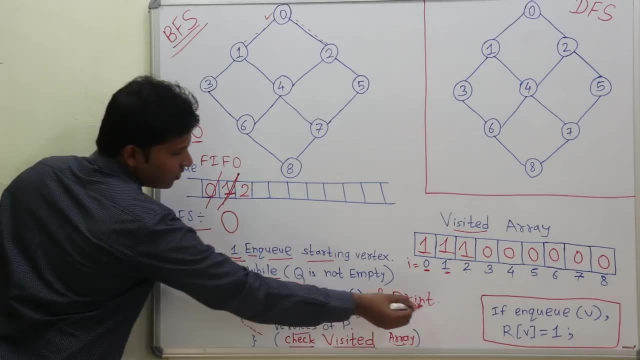 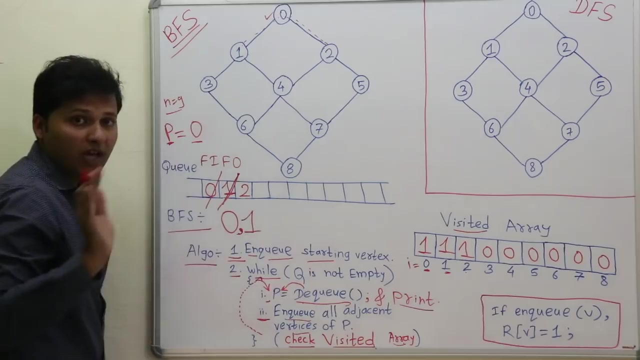 to dequeue. So now the next dequeuing vertex will be the vertex 1.. So the vertex 1 will be dequeued. So whenever you dequeue a node, you print that node As you are recording the BFS. the vertex 1 will be dequeued. So now you have to set the pointer p to vertex 1, because that is. 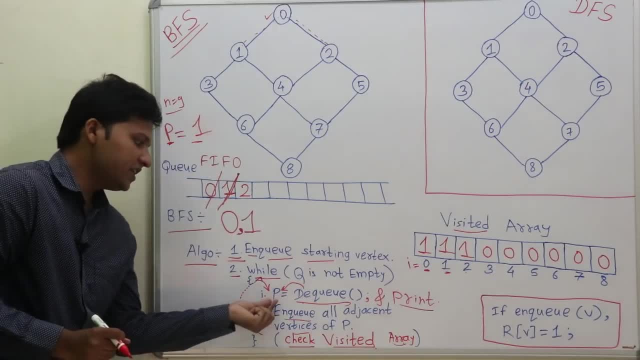 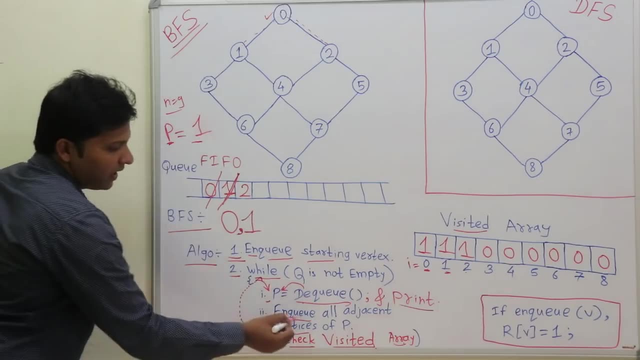 the dequeued vertex now. So, as it is written here, p is equal to dequeue, So p points to vertex 1 now. So now let us go to the second step: Enqueue all adjacent vertices of p. So what is the vertex? 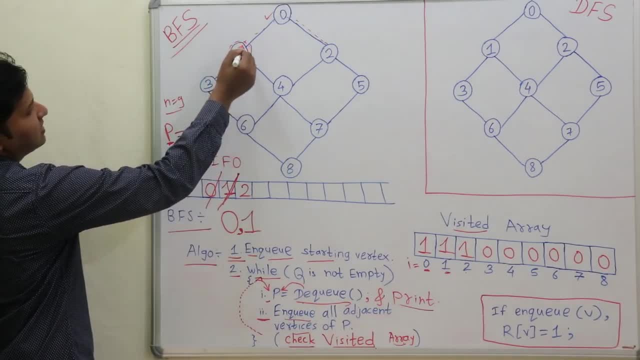 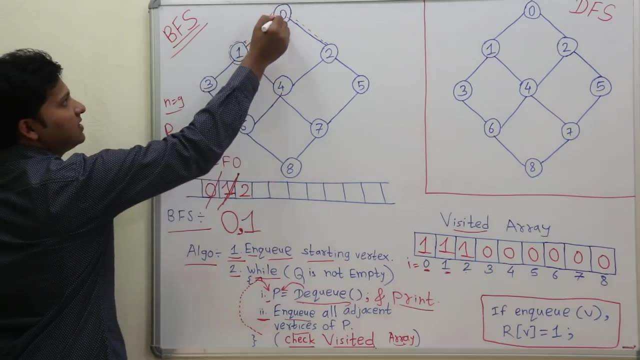 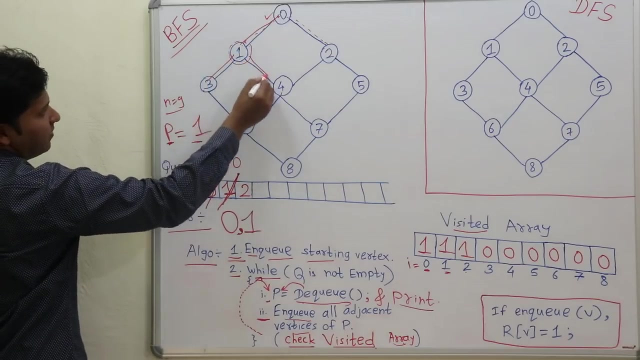 p, That is 1.. So what are the adjacent vertices for vertex 1?? So the adjacent vertices for vertex 1 are 3,, 4 and 0. So see here what are the adjacent vertices: That are 0,, 3 and 4.. So now, 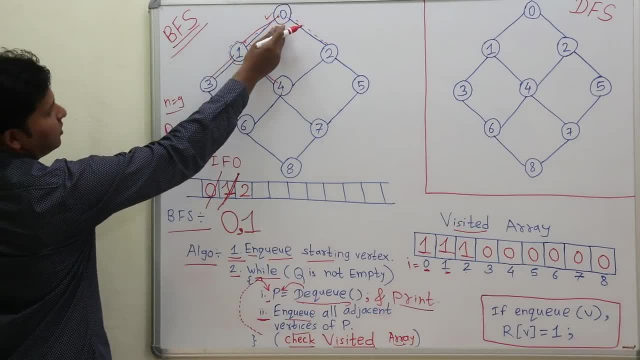 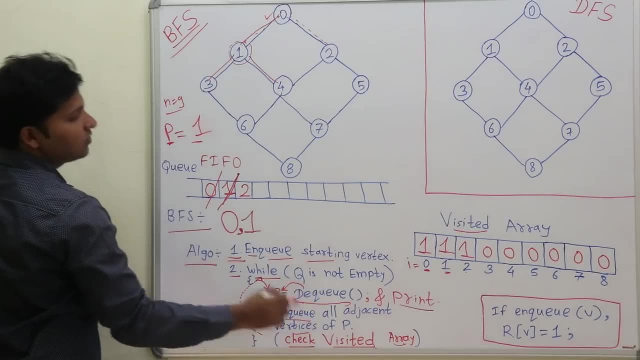 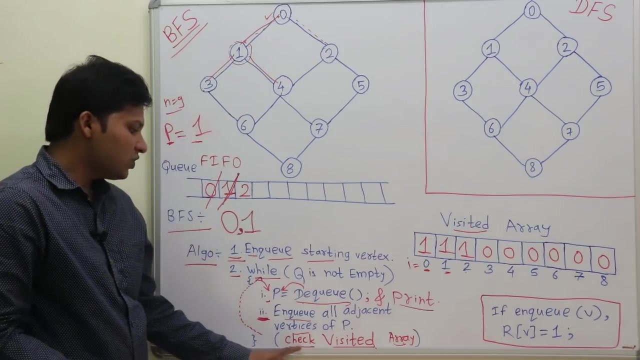 let us go one by one. So for vertex 0 can you enqueue that vertex? See as it is written here in the second step: enqueue all adjacent vertices. So can you enqueue vertex 0?? No, you cannot enqueue, because an extra condition is there. So you cannot enqueue that vertex. So you cannot enqueue. 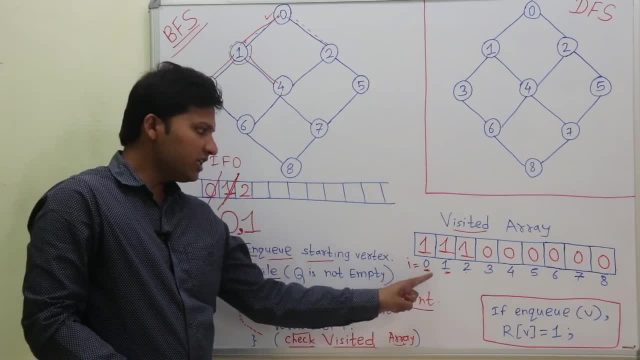 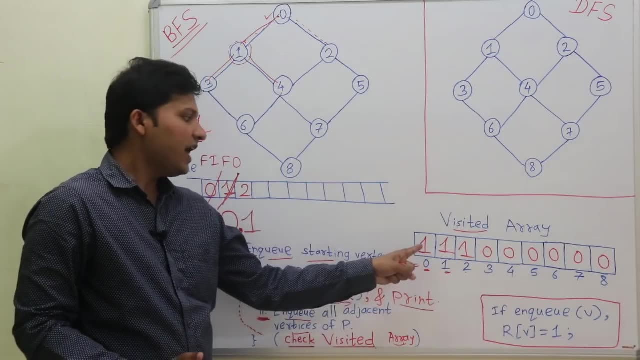 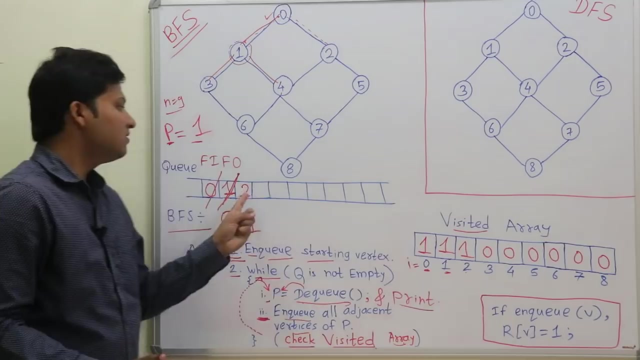 because an extra condition is to check the visited array. and when you check the visited array here- see for vertex 0- the flag is 1.. The flag is set here means it is already visited. So you cannot enter vertex 0 inside the queue again. So let us go to the next adjacent. 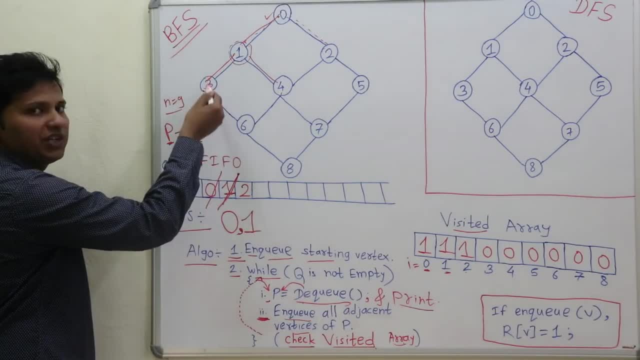 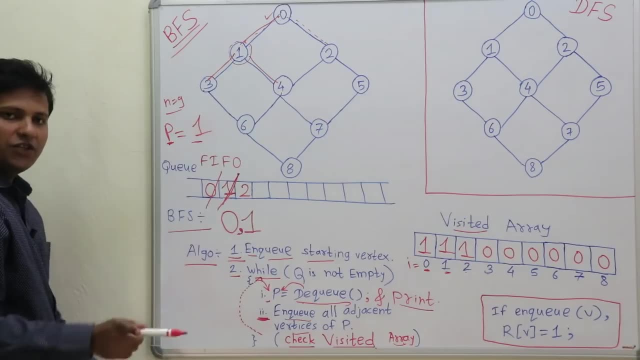 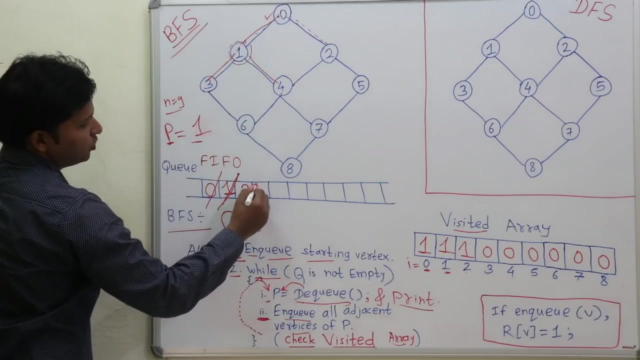 vertex. The next adjacent vertex is vertex 3.. Now for vertex 3. check inside the visited array. The value is 0 means that vertex is unvisited. So as the vertex is unvisited, you can enter that vertex inside the queue. and after you enter that vertex inside the queue, 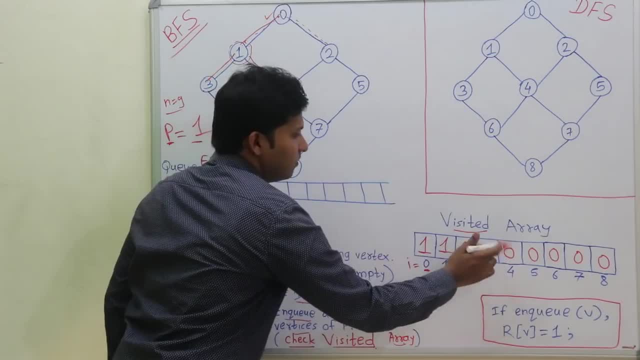 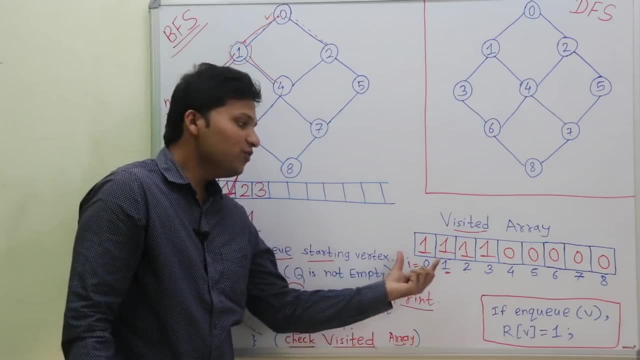 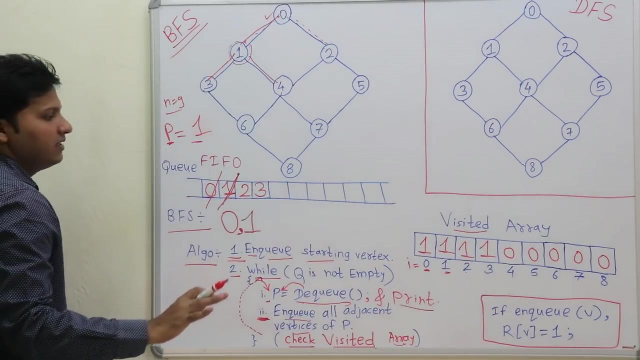 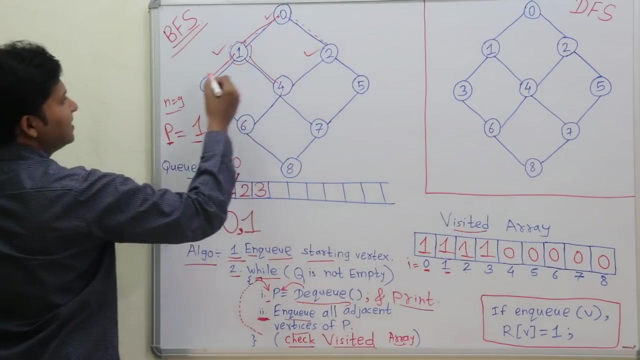 make the value 1 here, Right, Okay, Now I will tell you a shortcut trick. Now, if you are doing this on a paper, then it is not needed to write this visited array. Instead of setting the flags 1 inside this visited array, you can just mark these vertices as the right mark Means the. 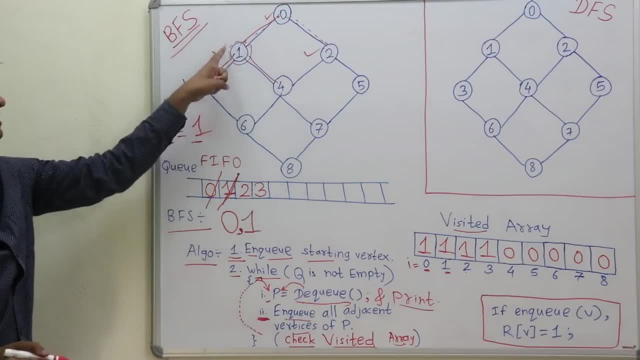 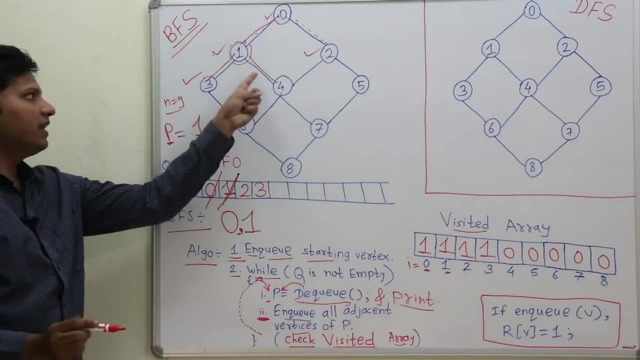 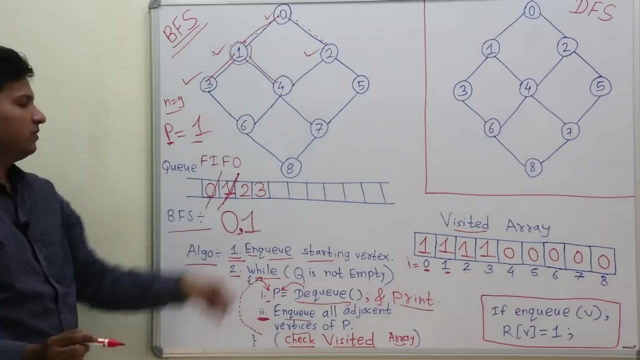 correct mark That means these vertices are visited. The flag for these vertices is 1.. Now let us go to the next adjacent vertex. The next adjacent vertex for 1.. 1 is 4. right, so check for 4. yes, it is yet unvisited, so you can enter that inside the. 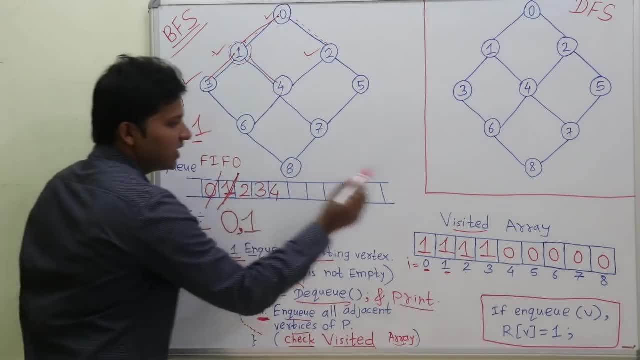 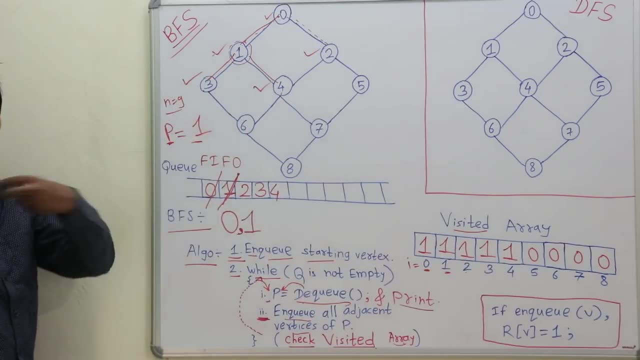 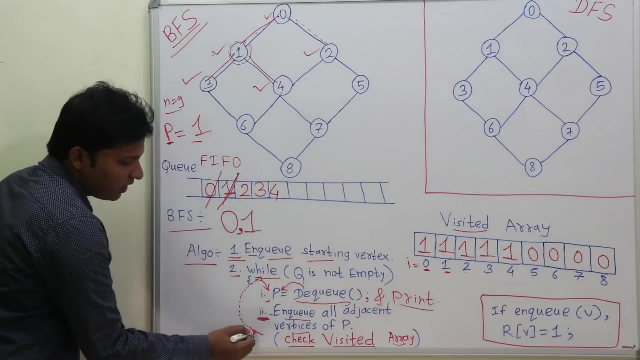 queue right, and after you enter that inside the queue, you have to make the value 1 in the visited array and just check it as visited. So now, as all the adjacent vertices are over, this step is over now and let's go to the next while iteration. Now, again, the queue is not empty, so go inside. 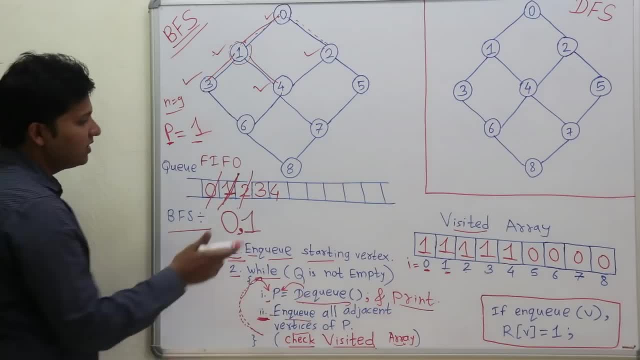 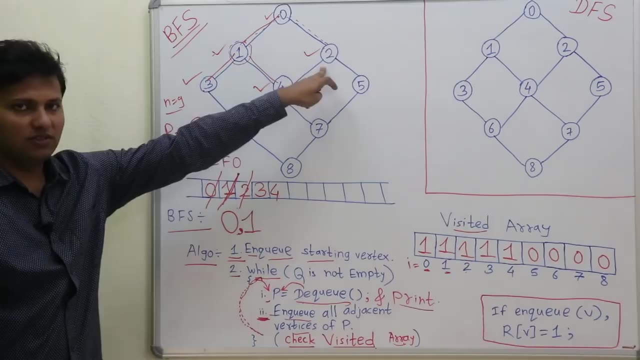 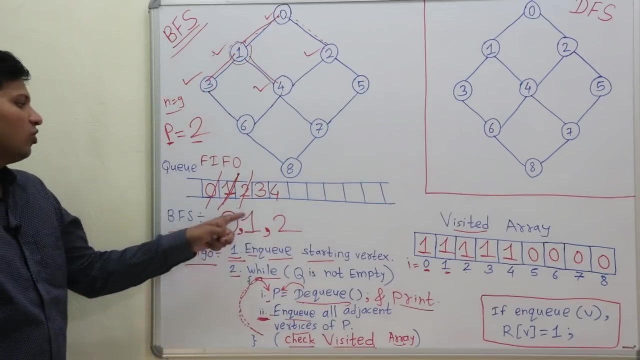 p is equal to dq. Now the next dequeuing vertex is the vertex 2. okay, so vertex 2 is dequeued now. so after you dequeue, you have to print it in the traversal. so 0, 1 and then 2 is printed. So now 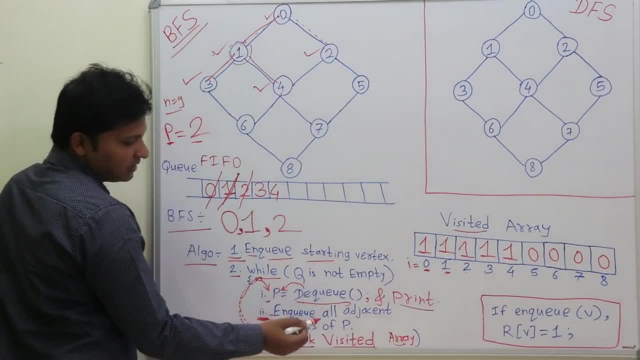 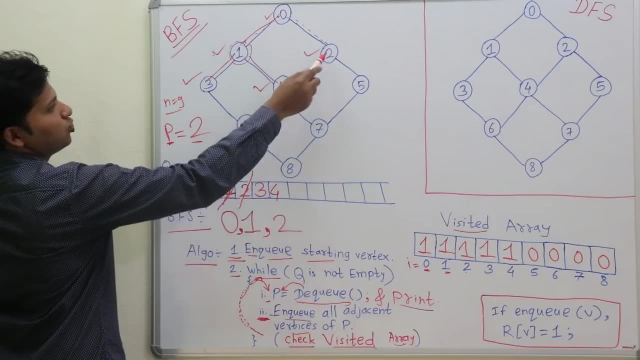 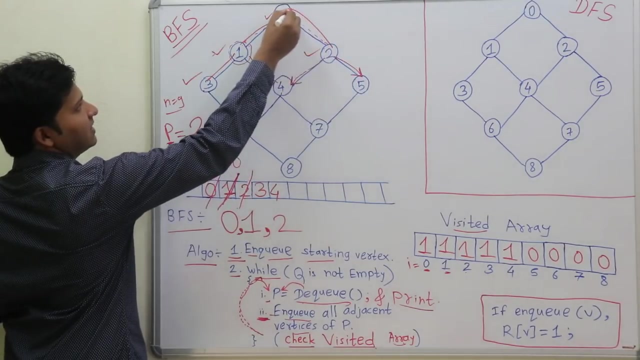 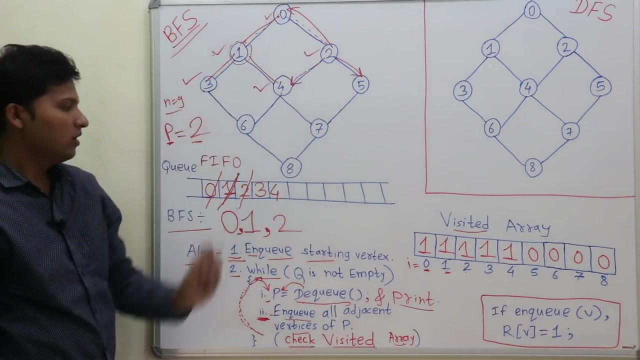 after this step is over, let's go to the second Step, that is, enqueue all adjacent vertex of p. so check adjacent vertices of vertex 2 c, vertex 4, then vertex 5 and then vertex 0. okay, so start 1 by 1. so at first check the adjacent vertex 0. so 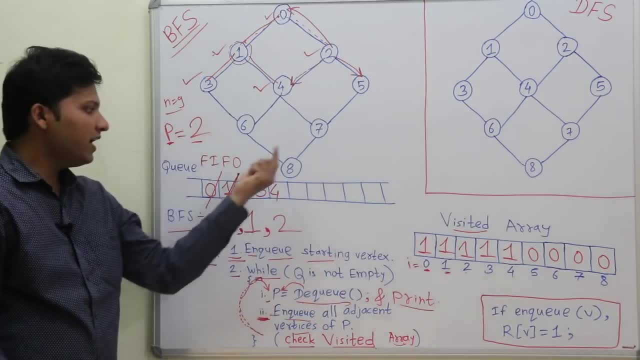 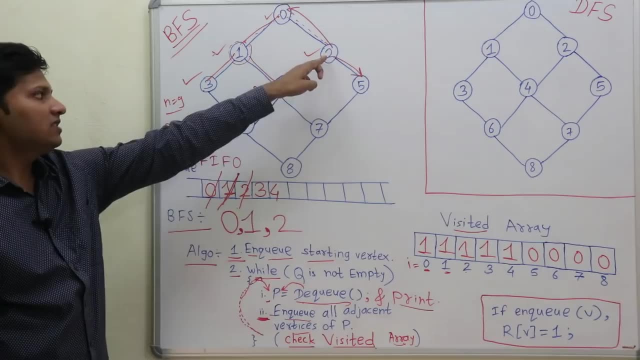 for adjacent vertex 0, the flag is set, so you cannot enter it again inside the queue. So now let's go to the next step, the second adjacent vertex. The second adjacent vertex for vertex 2 is the vertex 4.. So check. 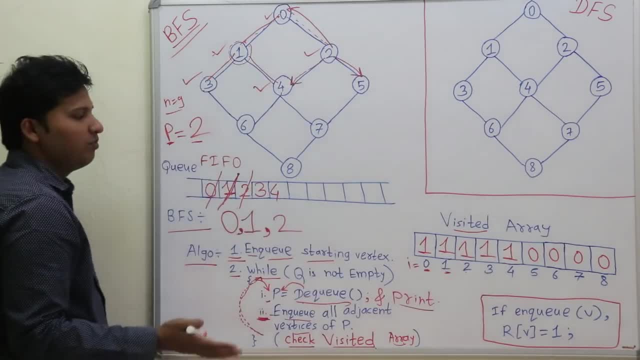 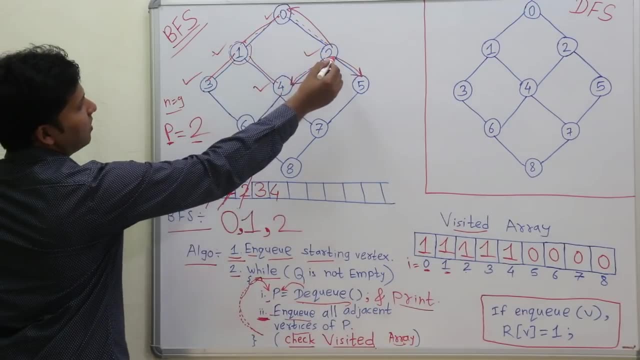 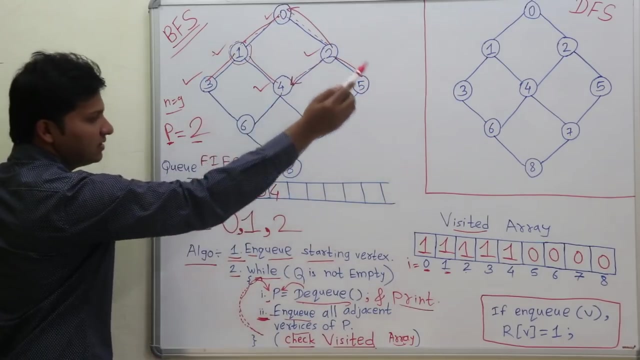 inside this visited array the flag is set means it is already visited, So you cannot enter inside the queue again. Now let us go to the next adjacent vertex. The next adjacent vertex is vertex 5.. So check inside the visited array. Yes, this vertex is yet unvisited because the value is: 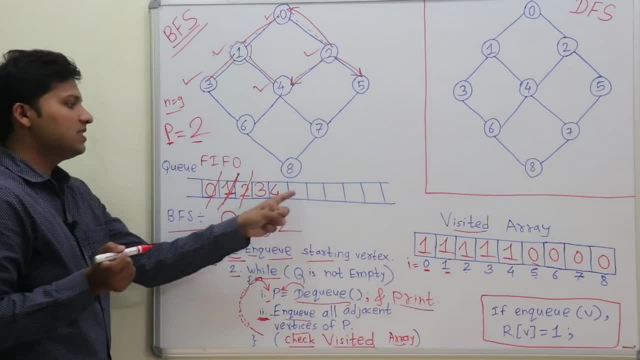 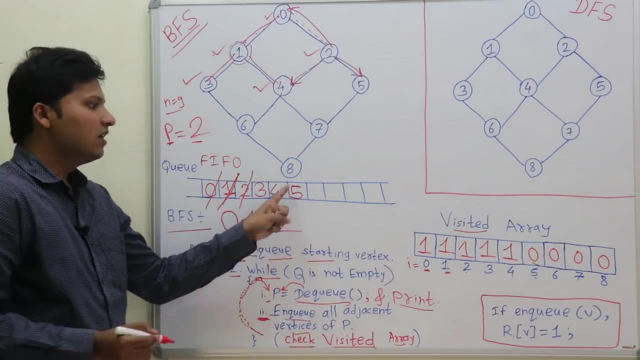 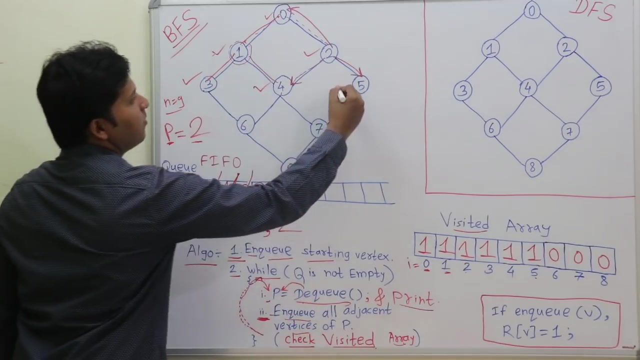 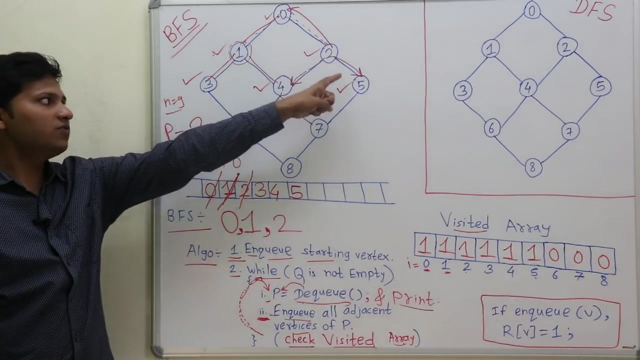 0. So you can enter this inside the queue. So I enqueue that vertex and when you enqueue that vertex you just set the flag as 1 for that vertex and just check mark. it means this vertex is now visited. So as all the adjacent vertices are over for vertex 2, let us go to the next while. 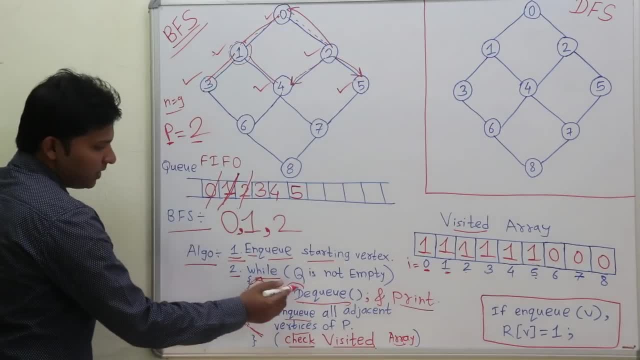 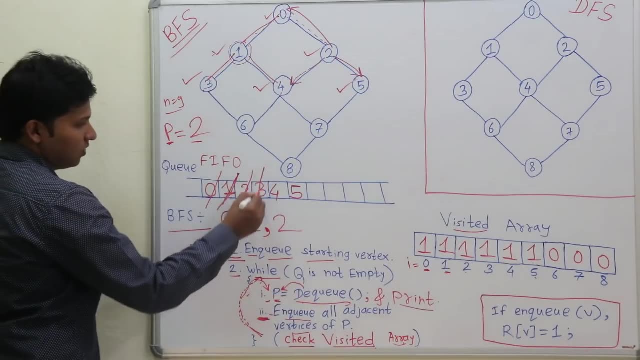 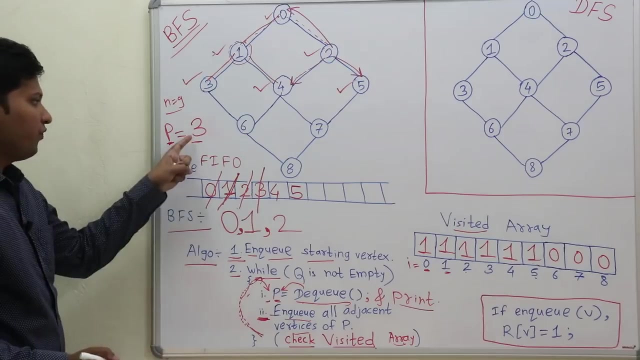 iteration means the next while loop. Now again, queue is not yet empty, So go inside. So p is equal to dq. So the next dq vertex is the vertex 3.. So for vertex 3, now you have to. 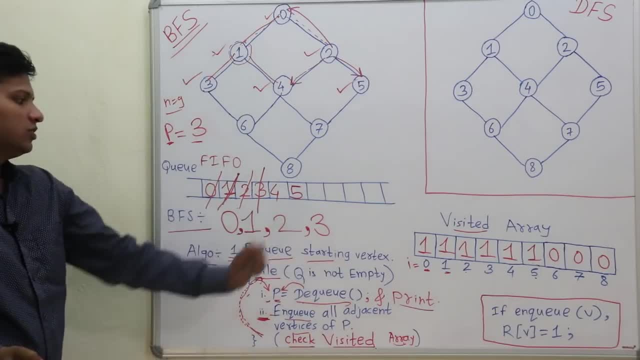 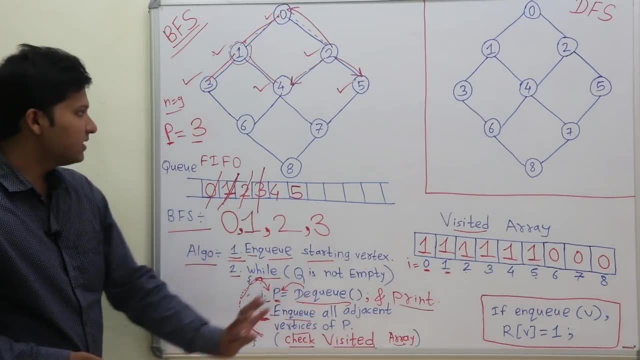 print it in The bfs traversal. So you have printed 3.. So after you print 3, let us go to the next step. Enqueue all adjacent vertices of p means that is the vertex 3.. So what are adjacent vertices of? 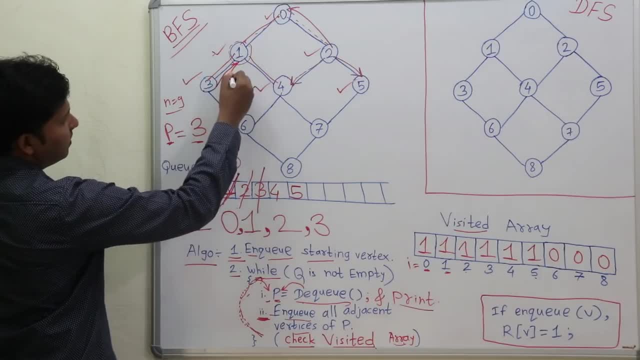 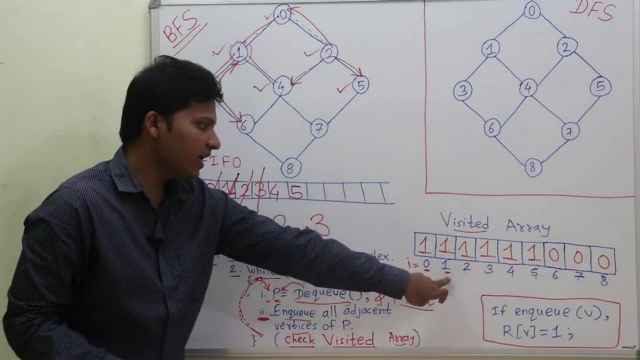 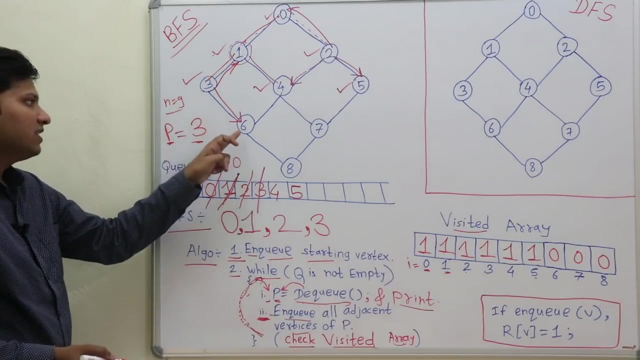 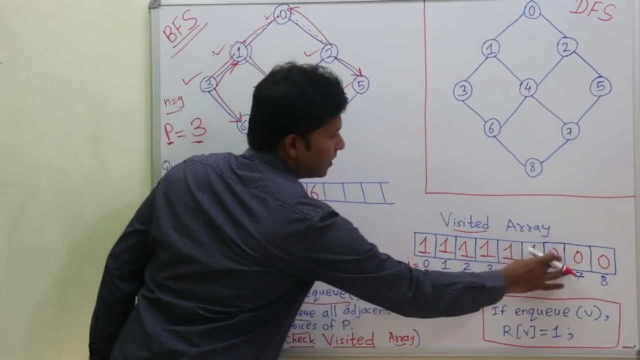 vertex 3 now See vertex 1 and vertex 6.. So let us go one by one. So for vertex 1,, the visited array, the flag is set, So you cannot enter again Now. the next adjacent vertex is vertex 6.. That is yet unvisited. So enqueue that vertex and set the 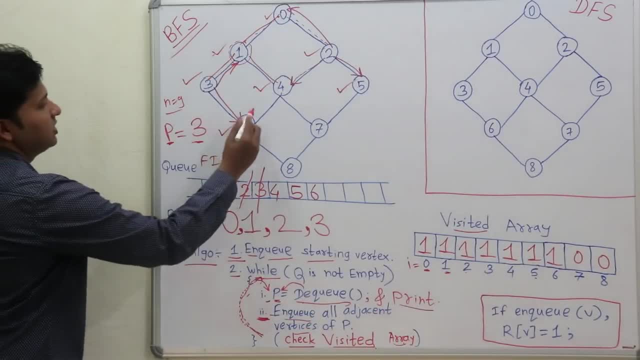 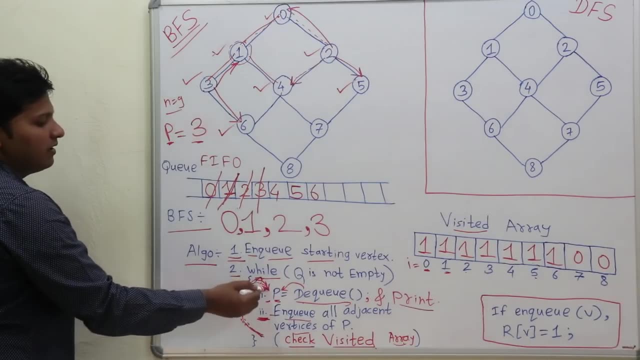 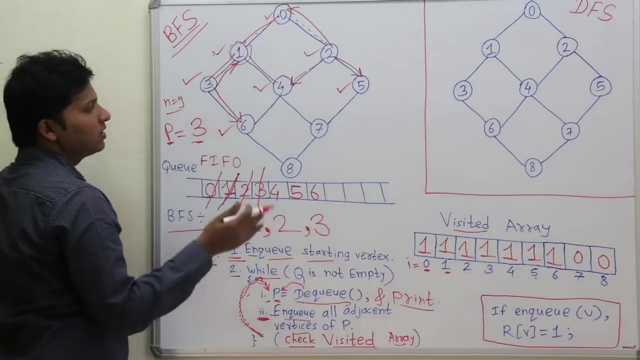 flag as 1 and check it means that vertex is visited. So all the adjacent vertices are visited. Let us go to the next iteration Now. I will do it fast. I will not go inside this code now, As you remember the code now, So see. 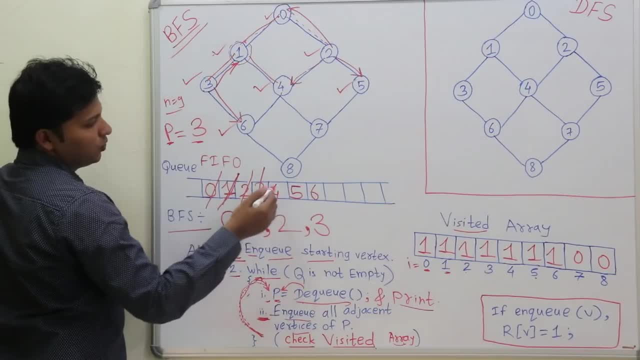 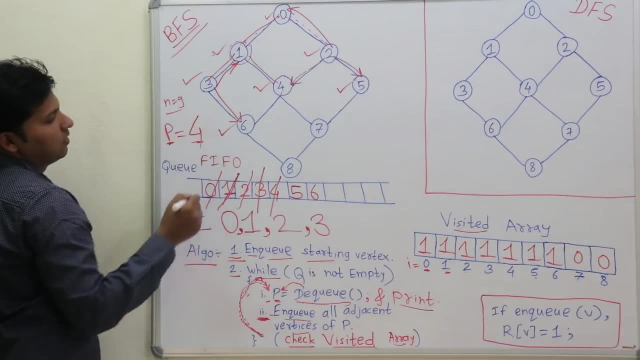 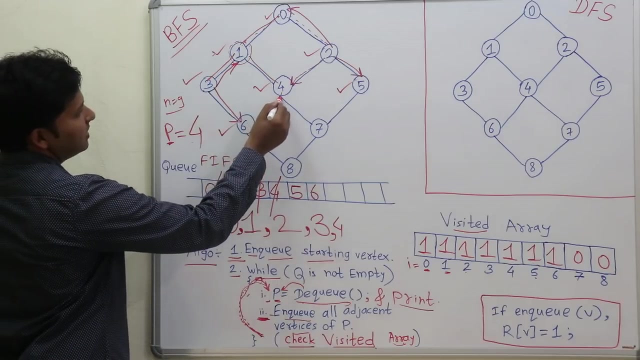 as the q is not yet empty, dequeue. So when you dequeue now, the next dequeued vertex is vertex 4.. So for vertex 4, you have to print it in the traversal. After you print, check all the adjacent vertices of vertex 4.. So what are the adjacent vertices? See vertex 6,, vertex 7,. 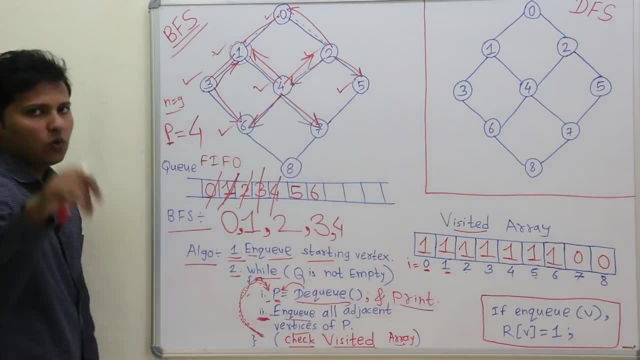 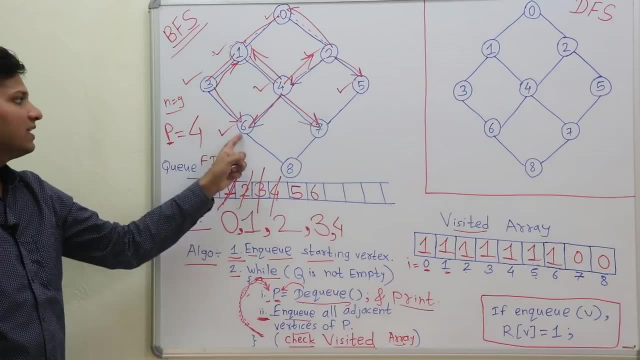 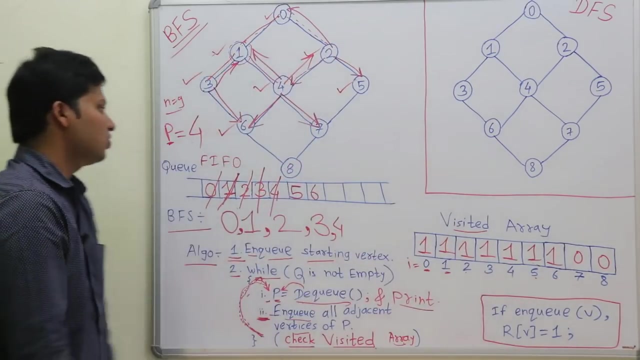 vertex 1 and vertex 2.. So let us go one by one. Vertex 1 is visited. Vertex 2 is already visited. Now, vertex 6 is already visited. Vertex 7, yes, it is yet unvisited. So enqueue that vertex. 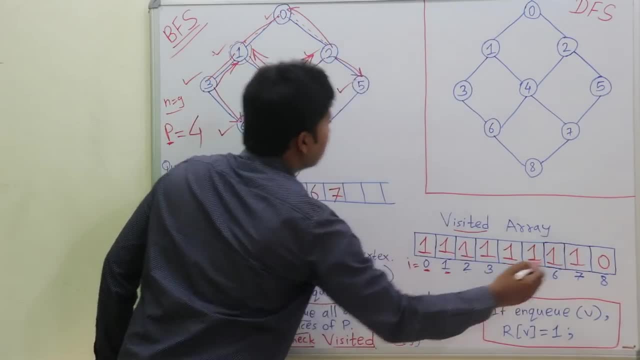 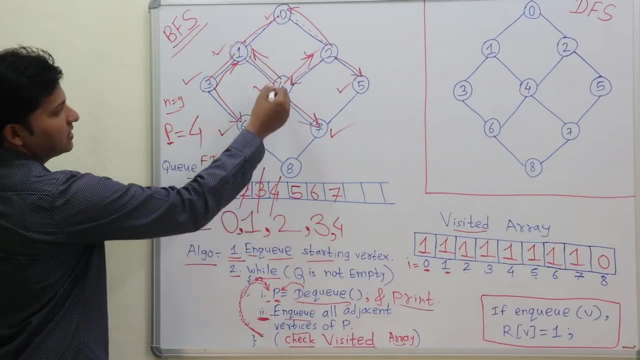 set the flag as 1 and just check it Means that vertex is now visited. Now, as always, let us go one by one. So let us go one by one. So let us go one by one. So all the adjacent vertices for vertex 4 are over, So let us go to the next while loop, So inside. 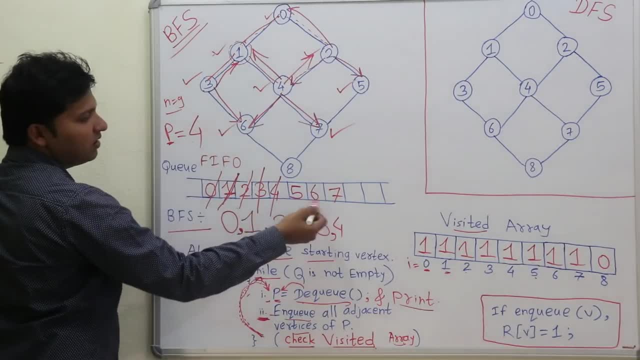 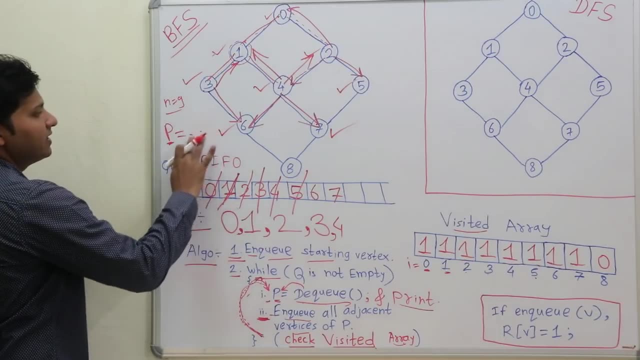 the next while loop you have to check whether the q is empty. No, it is not empty, So go inside and dequeue. So when you dequeue now, the dequeued vertex is vertex 5, and after you dequeue you have. 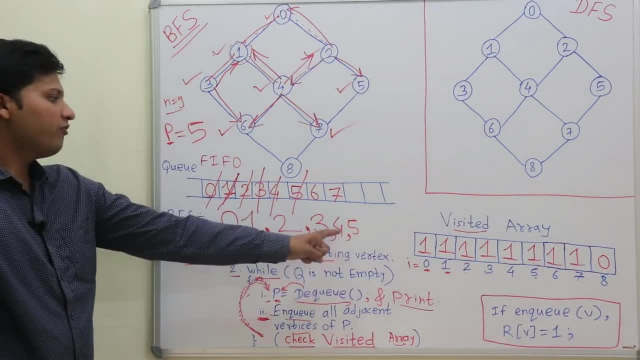 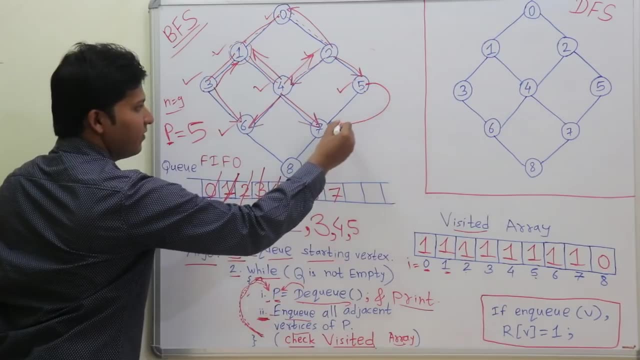 to print it. Okay, now you have printed it, So you have to check the adjacent vertices. So the adjacent vertices are vertex 7 and vertex 2.. Okay, So let us go one by one For vertex 2,. 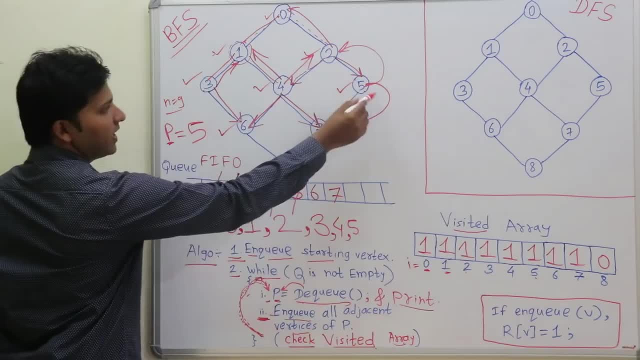 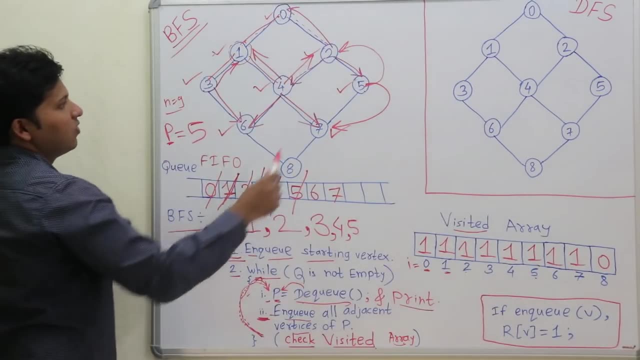 the flag is set. So it is visited. Now let us go to the next adjacent vertex. So the vertex is 7.. Vertex 7 is also visited. So both vertices are visited. So nothing is to be enqueued. Okay So, 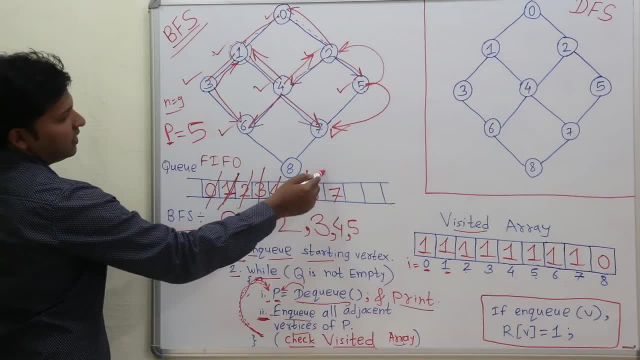 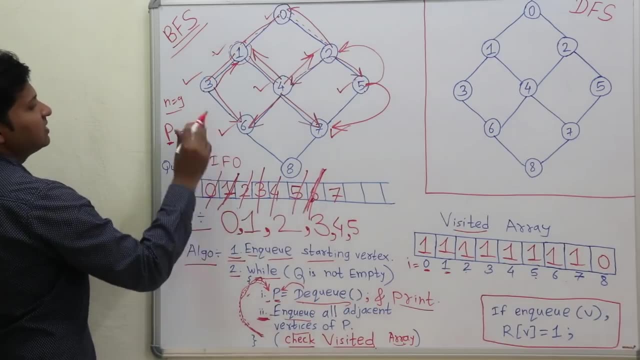 let us go to the next while loop. So in the next while loop, check whether the q is not empty. No, it is not empty, So dequeue. So the next dequeued vertex is vertex 6.. So for vertex 6, print it in the 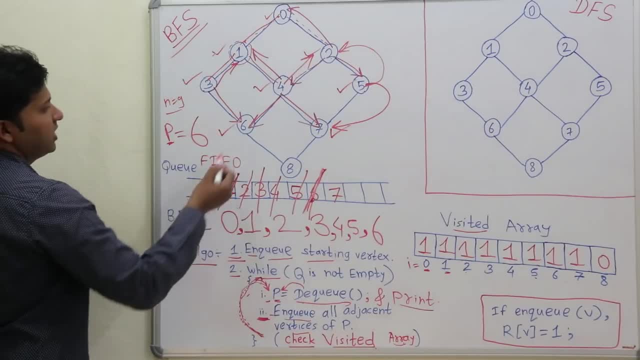 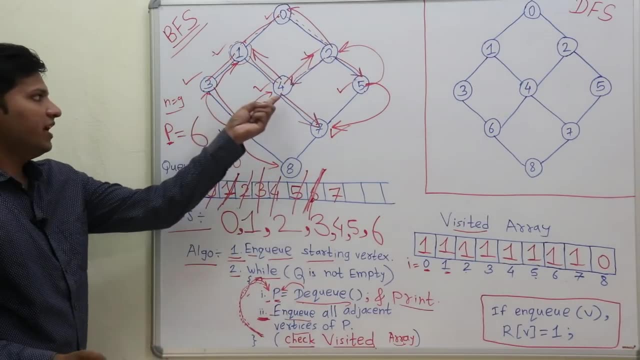 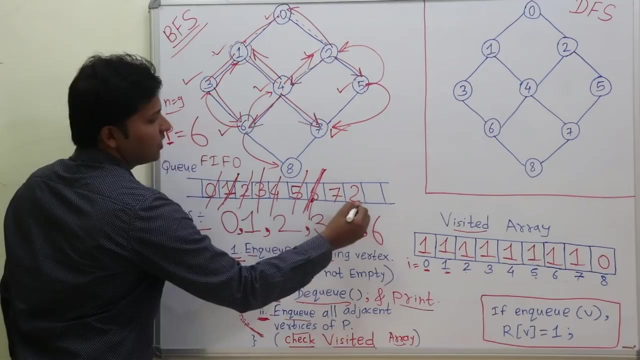 BFS traversal. Now check the adjacent vertices: See vertex 3, vertex 4 and vertex 8.. So 3 and 4 are visited already. Only vertex 8 is yet unvisited. So enqueue that vertex And after: 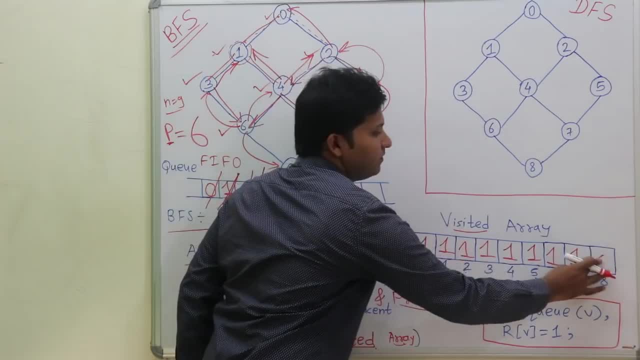 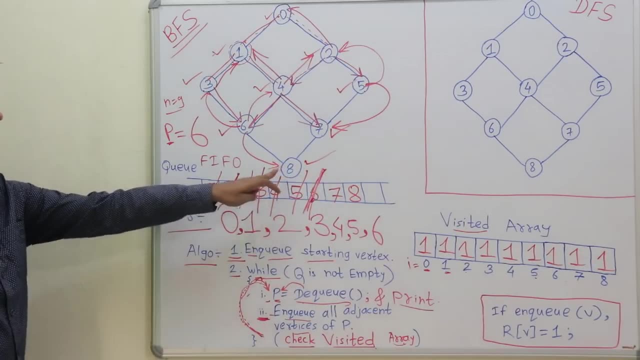 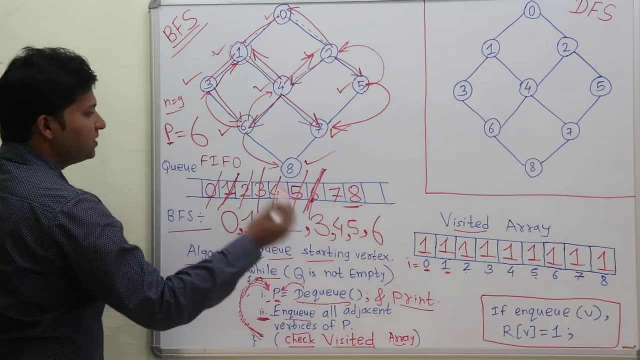 you enqueue a vertex, you have to set the flag as 1, and when you set the flag 1, you just checkmark it right. let's go to the next while loop. so for the next while loop, check whether the queue is not empty. no, it is not empty, so go inside and dequeue. so the next dequeued vertex is vertex 7. 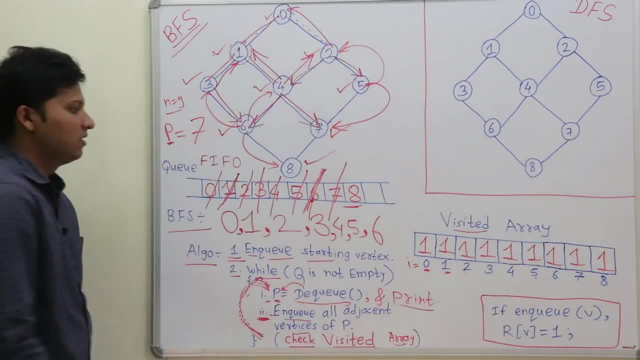 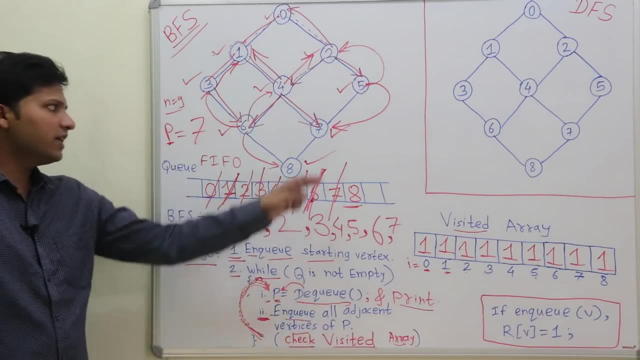 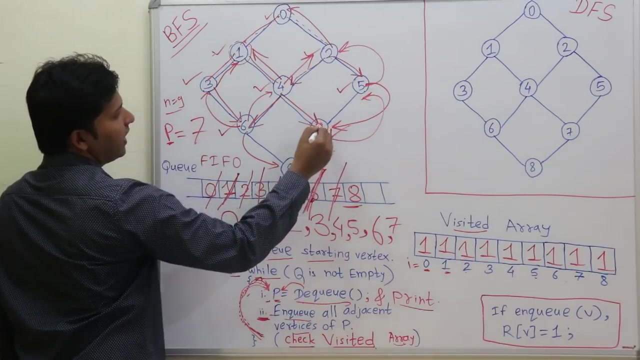 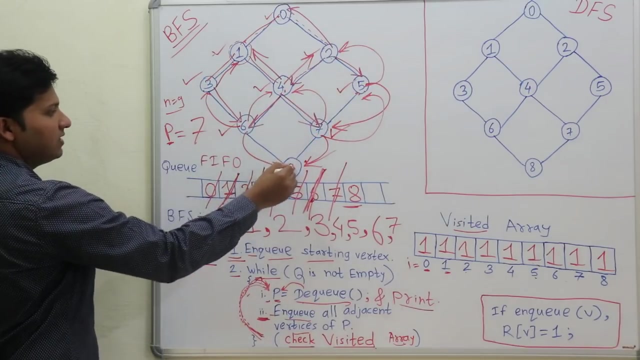 so check here, vertex 7 and print it. so after you print it, go for all the adjacent vertices of vertex 7. now for vertex 7. the adjacent vertices are vertex 8, vertex 5 and vertex 4. right, so let's go one by one. 4 and 5 are already visited and 8 is also visited, so nothing is to be enqueued. and 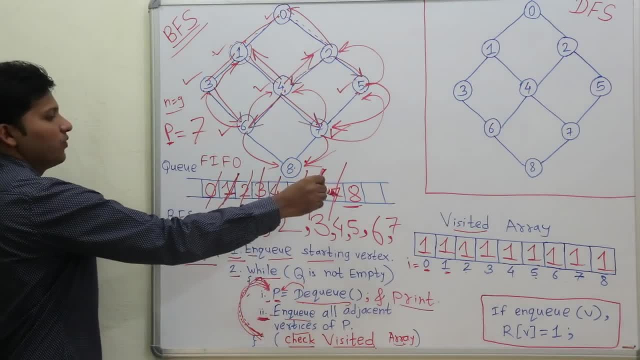 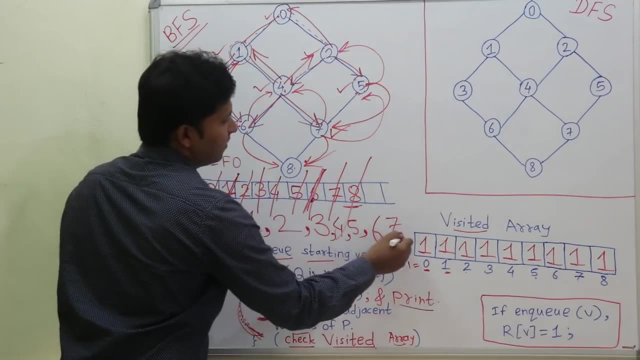 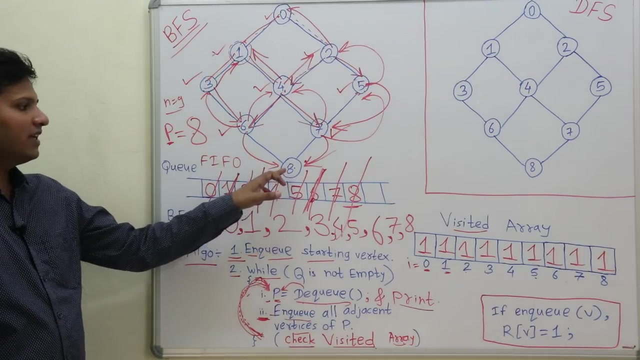 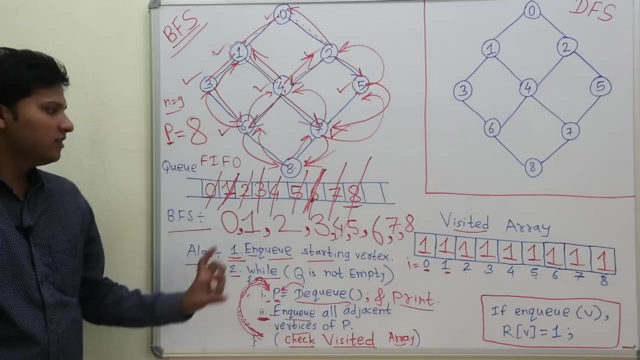 go to the next while loop now. so when you go to the next while loop you dequeue. so now the dequeued vertex is vertex 8 and print it right. so after you print 8, now check all the adjacent vertices for vertex 8. so adjacent vertices are vertex 6 and vertex 7, but 6 and 7 is already visited, so nothing is to be enqueued. so 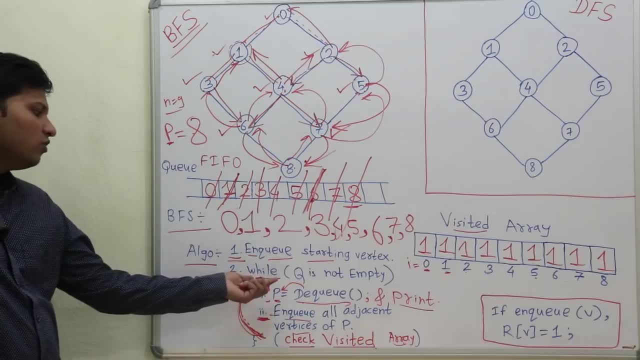 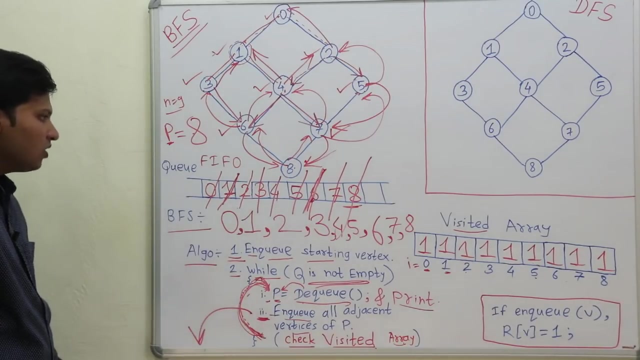 let's go to the next while loop. so where in next while loop you check while queue is not empty. but here the queue is empty. so this while condition is not satisfied and you come out of this while condition. okay, you come out of this while block. that means the bfs is. 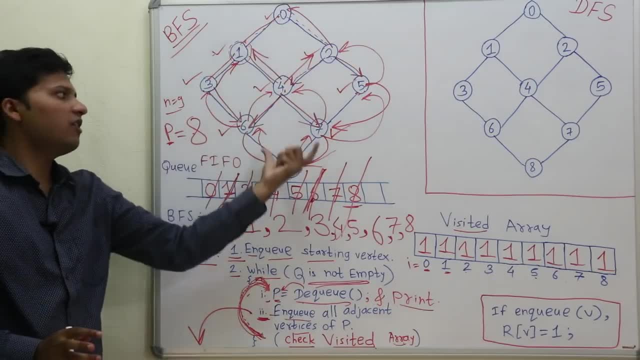 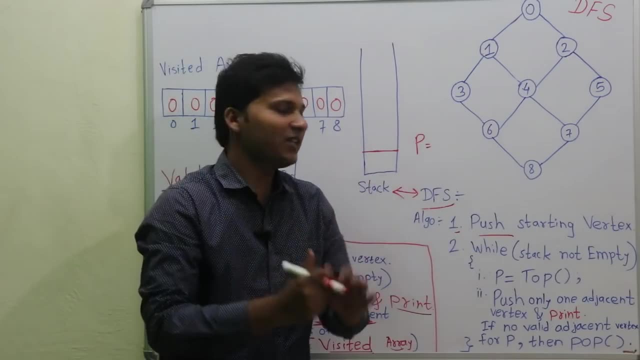 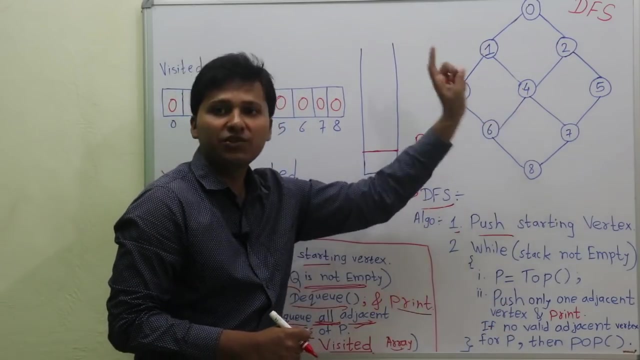 printed. the whole bfs for this graph is printed. now let's go and see how dfs works. so let's go for a dfs now. so here is the dfs algorithm and we are going to apply this DFS algorithm on this graph. So, while we apply this DFS algorithm, we are going to 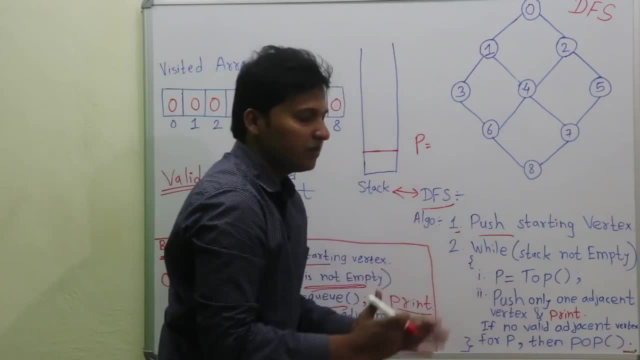 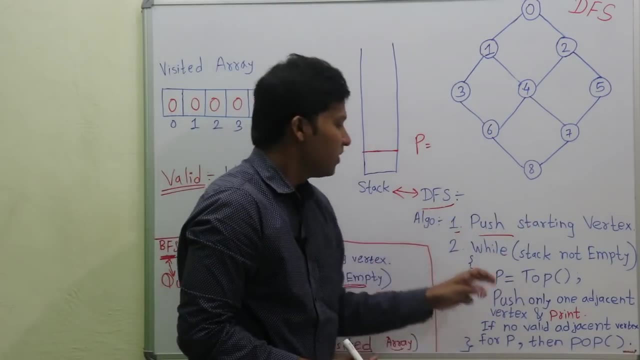 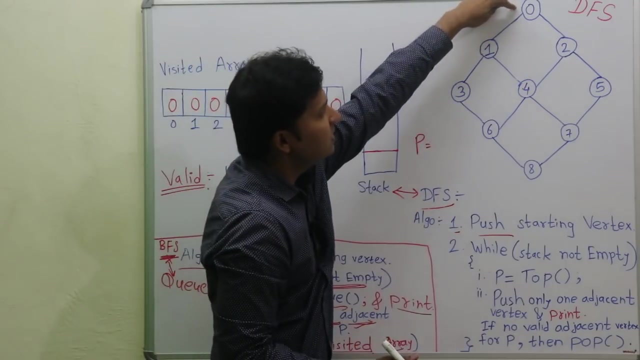 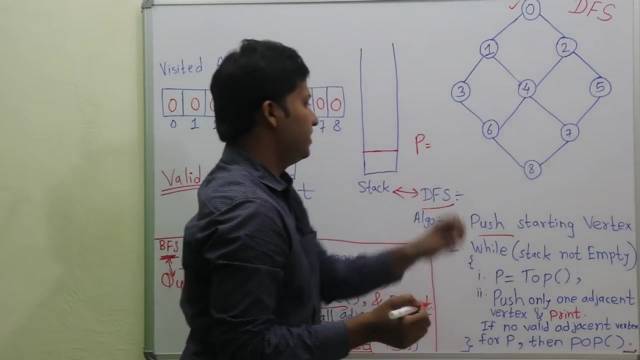 compare the BFS and this DFS algorithm. We are going to see the differences. So let us follow the steps of DFS algorithm. See, the first step is push starting vertex. So what is the starting vertex? here, See, we decide the starting vertex as 0. So 0 is the starting vertex. So push that. 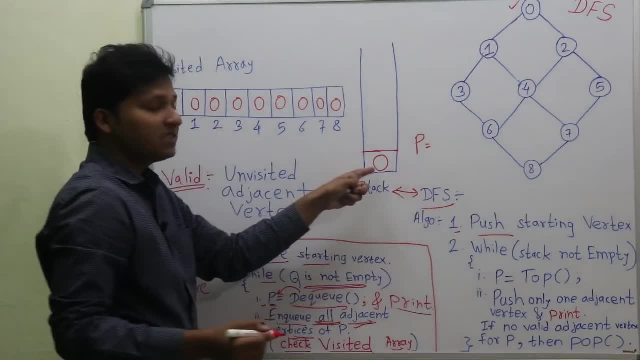 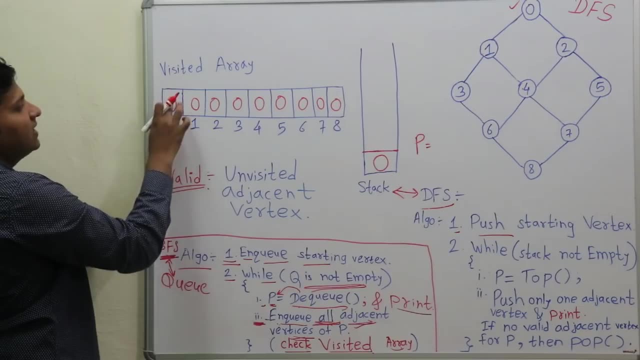 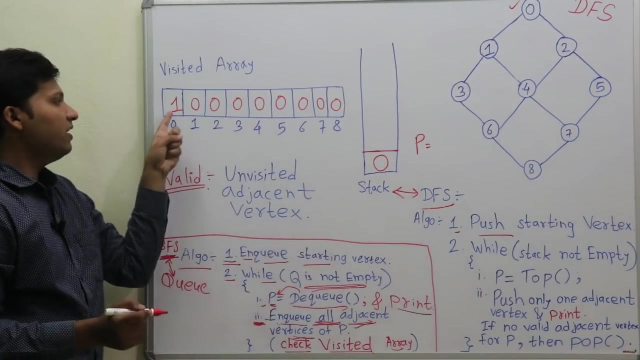 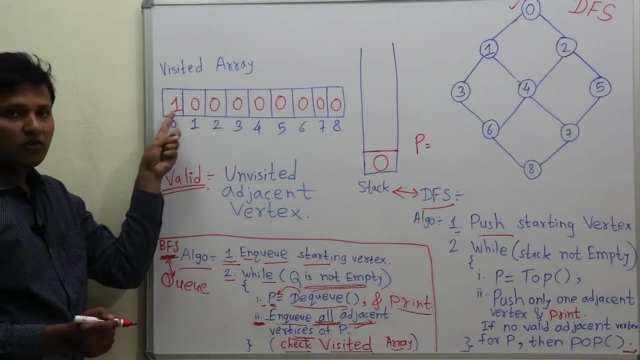 starting vertex here. So I push the starting vertex 0 and I set the flag for that starting vertex as 1, because, as it is pushed in the stack, it is now visited. So I make the flag as 1. To indicate that the vertex 0 is now visited. This is the visited array here. Now let us see. 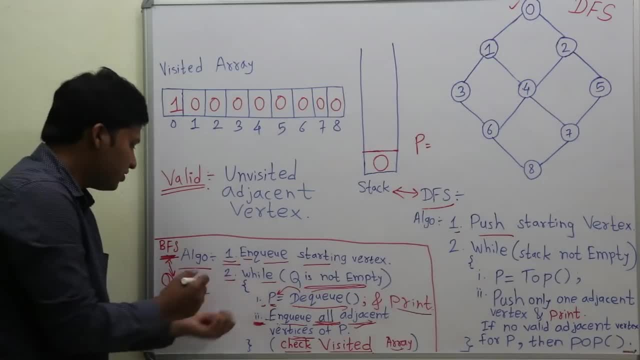 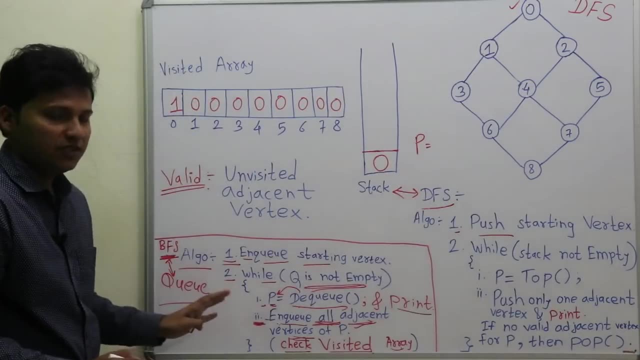 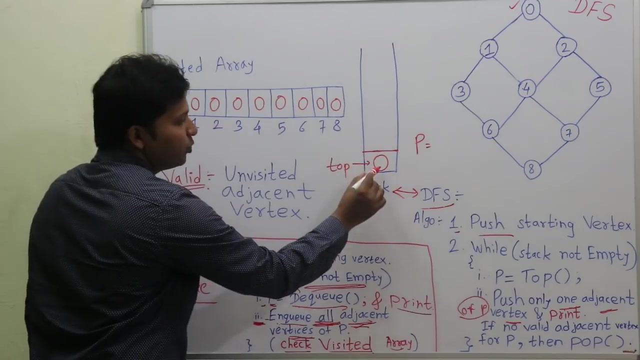 the difference. See, for BFS we use a queue and for DFS we use a stack. That is the difference. So now, whenever you push an element, you have to print that element. So you have pushed 0. Now you print that 0 in the DFS. 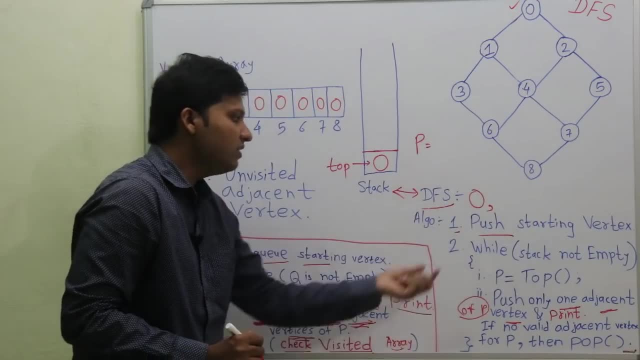 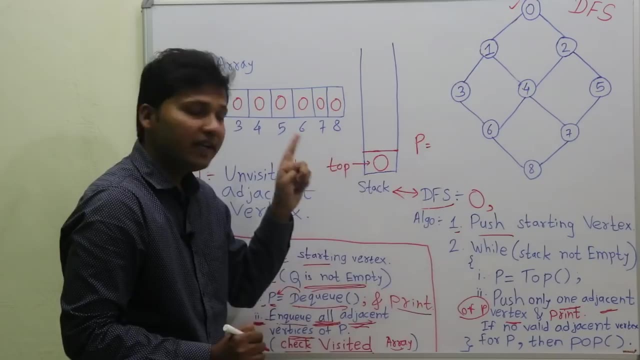 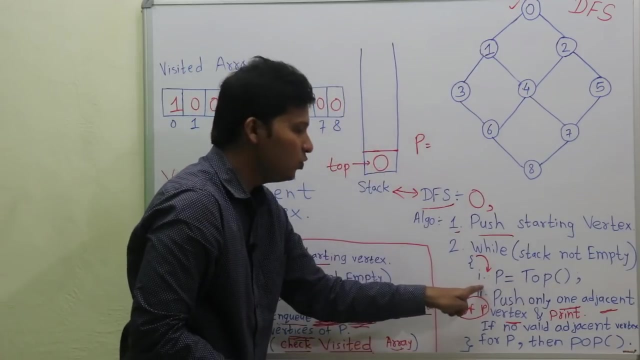 So, after you print that element, let us go to the second step. So now, while stack not empty. Yes, the stack is not empty. There is one element in the stack. So let us go to the first step. inside this, while loop, P is equal to top, So that means the top element of the stack. 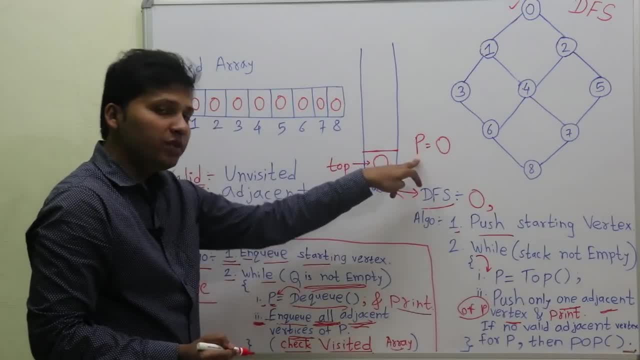 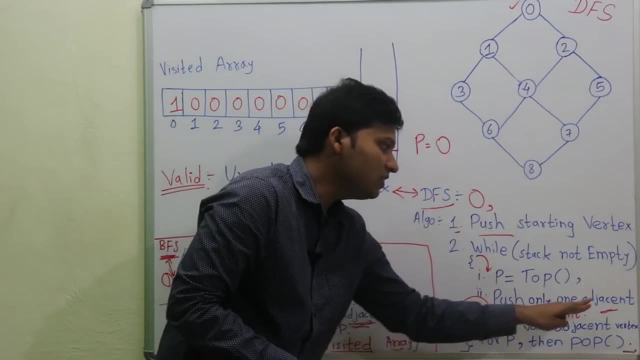 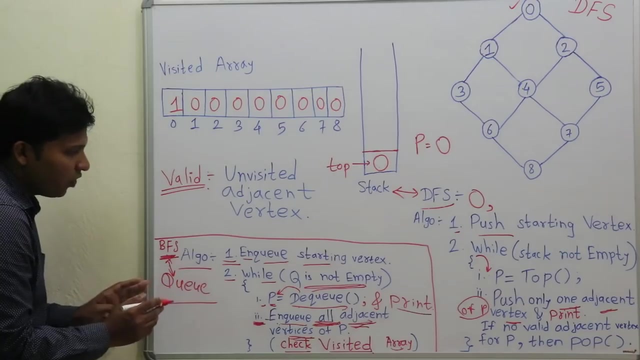 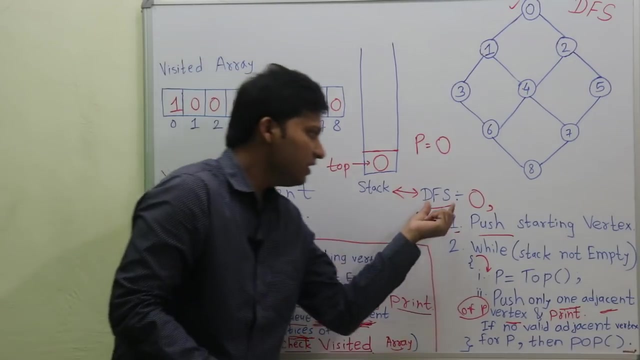 is assigned to P. So now P points to vertex 0.. So now the second step is: push only one adjacent vertex and print. So see here. Here is the difference. now See for BFS algorithm. we enqueue all adjacent vertices at a time, But in DFS 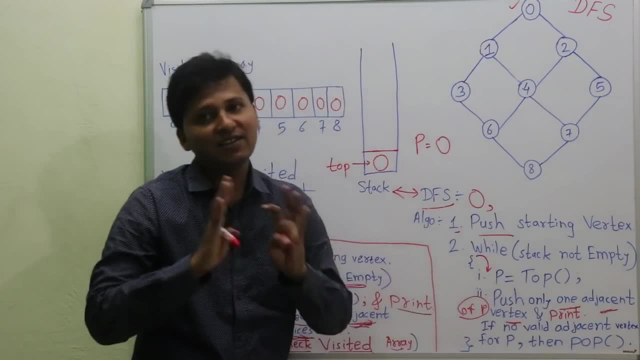 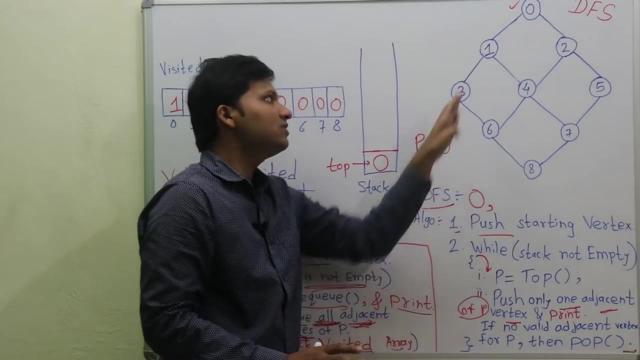 we push only one adjacent vertex at a time. So now let us see how many adjacent vertices are there for vertex P. So we push only one vertex at a time. See, there are two adjacent vertices, That is vertex 1, and 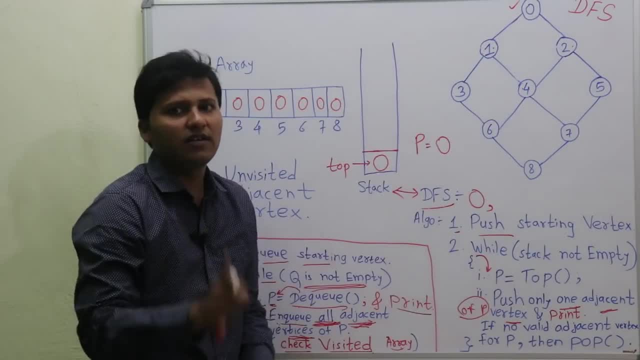 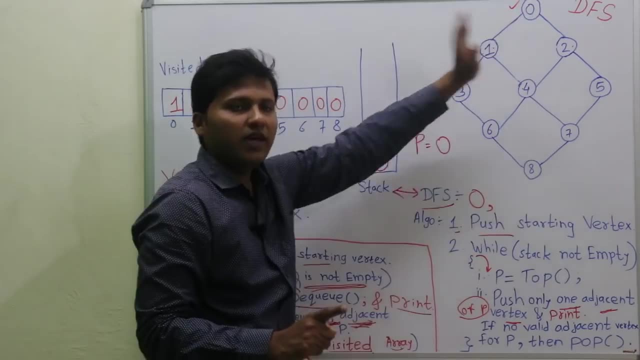 vertex 2.. So you can proceed with any one vertex, But you have to push only one vertex out of them. So you push either one or two, So I proceed with vertex 1.. So see, push one vertex, So I push. 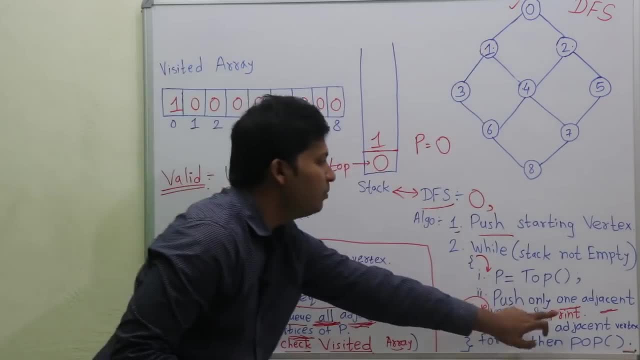 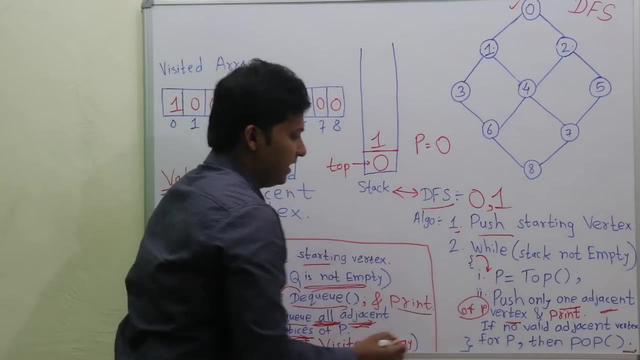 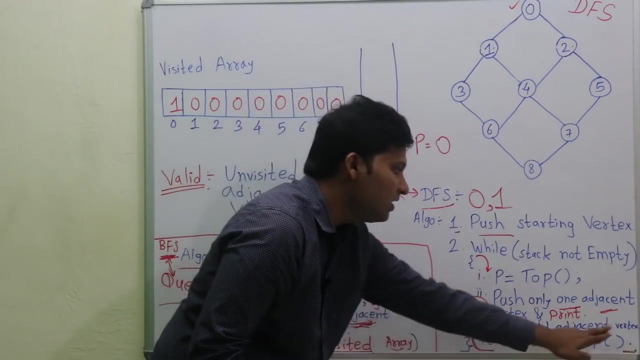 vertex 1 in the stack and I print that in the DFS record. So now there is one check condition for that. See, here is the condition. So what is the condition? If no valid adjacent vertex for P, then pop. So here was the condition of checking. visited. 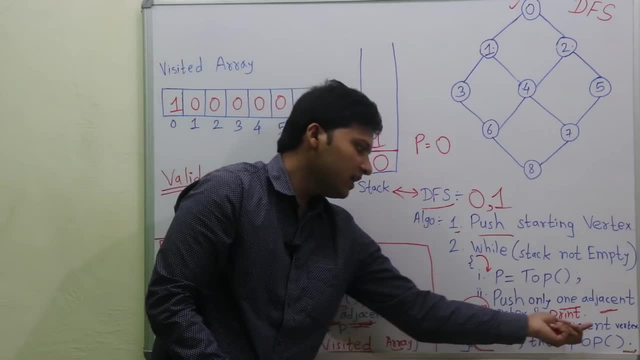 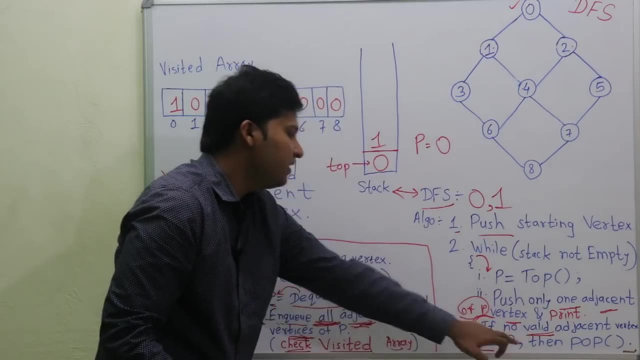 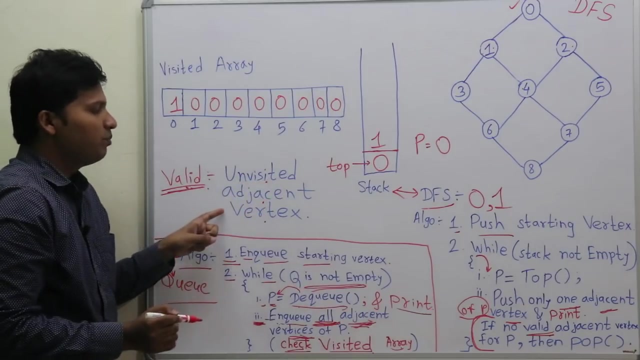 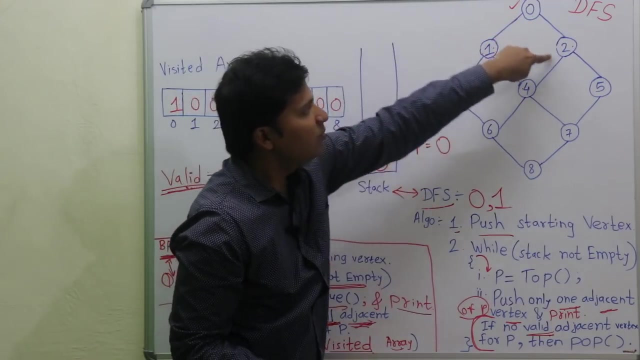 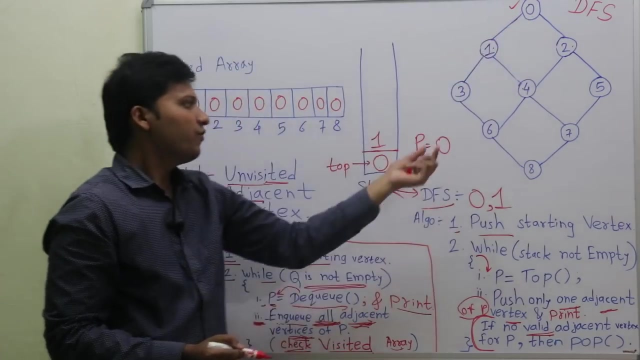 array And here is the condition of valid adjacent vertex. So what is a valid adjacent vertex? So I have defined it here, See: The valid adjacent vertex is the unvisited adjacent vertex. Means suppose there is vertex 0 and there are vertices available which are unvisited and adjacent to vertex 0. So for 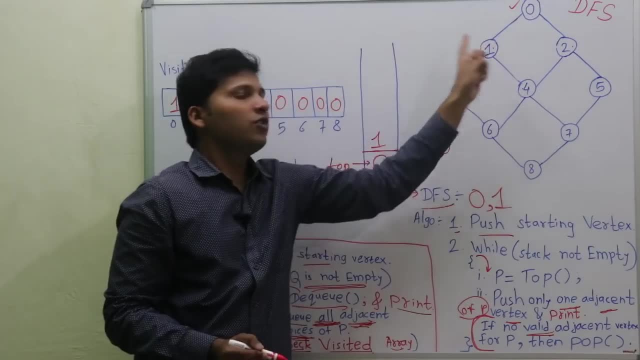 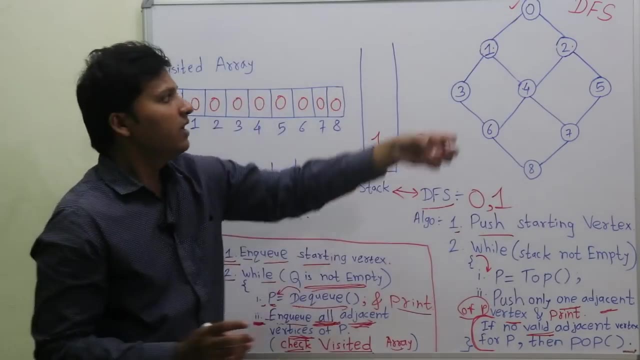 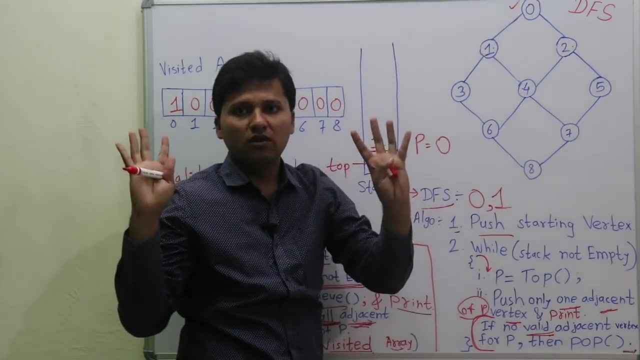 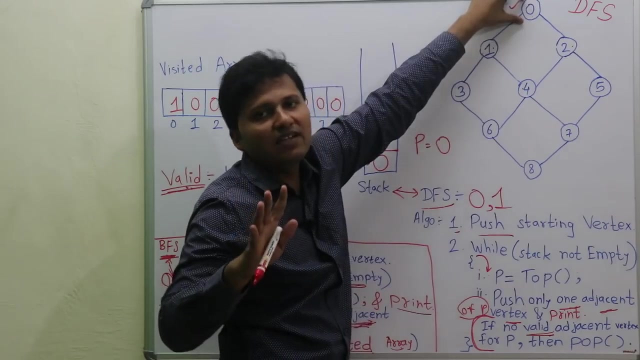 vertex P, there are vertices available which are unvisited and adjacent to that vertex. But just imagine If there are no vertices available for vertex 0, the vertex 0 is alone Means there is no valid adjacent vertex available for vertex 0. If that is the situation, then you have to pop the top element from the stack. 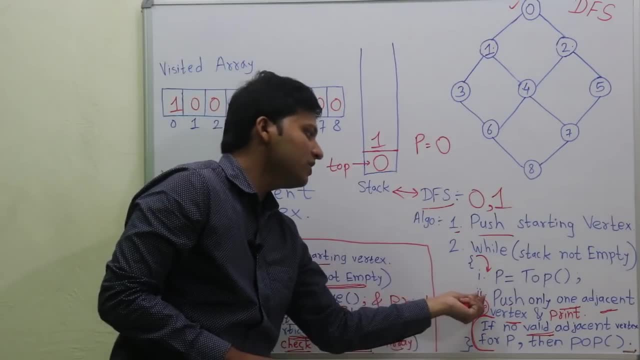 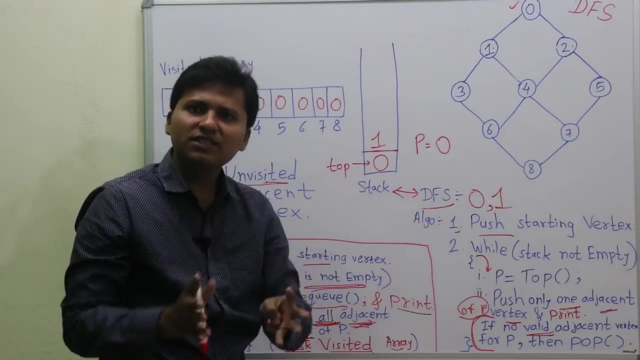 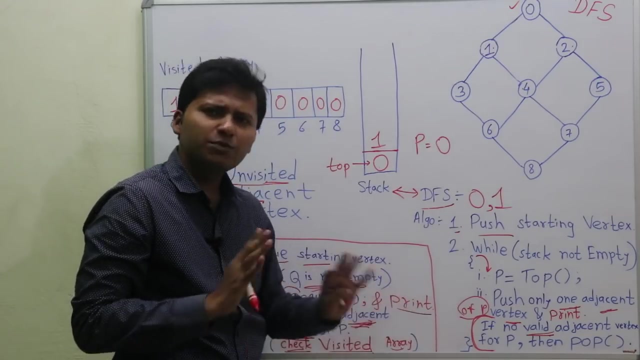 That is the checking condition here. So while performing the second step, you have to check this condition. Okay, This is a very easy condition. This is very simple. As we proceed further, you will perfectly understand this. Okay, There is no need to check this explicitly. 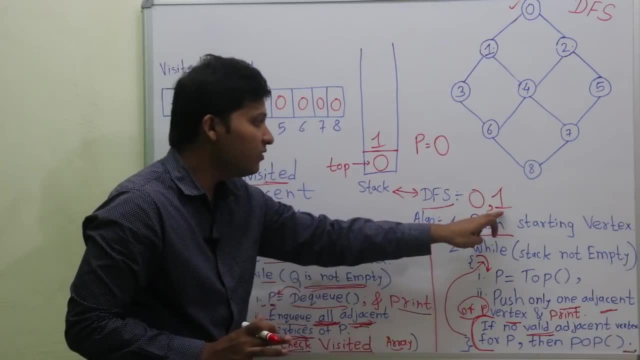 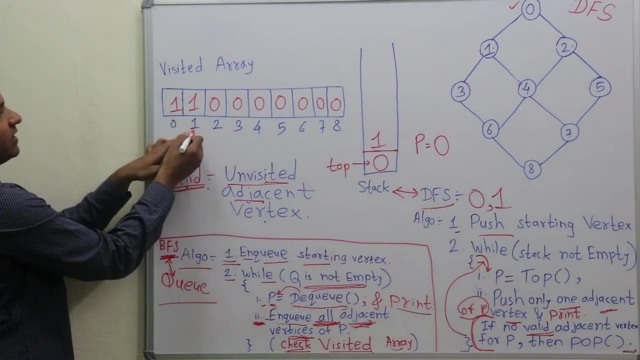 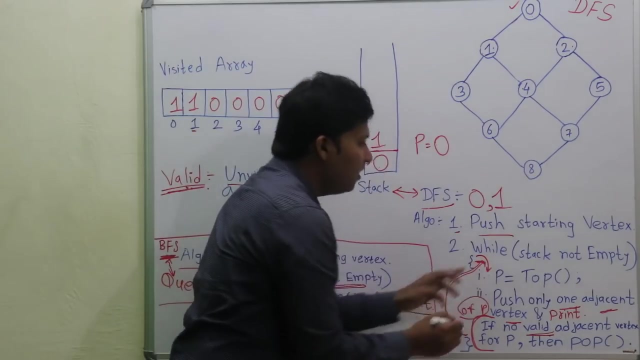 Automatically this happens. So now, as you have printed 1 and pushed 1 in the stack, that means you have to set the flag as 1 here. Okay For vertex 1, because now this vertex is visited. Okay, So now let's go to the next while loop. 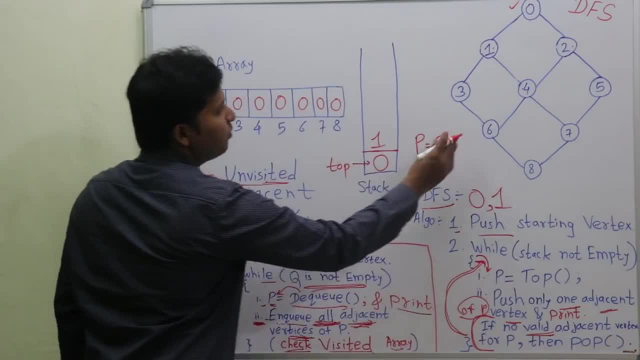 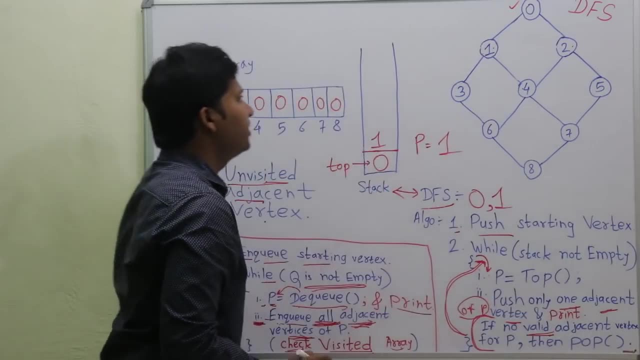 So here P is equal to top Is the first step. So now P points to vertex 1.. Okay, See, now push only 1 adjacent vertex and print: So for vertex 1, what is the adjacent vertex? 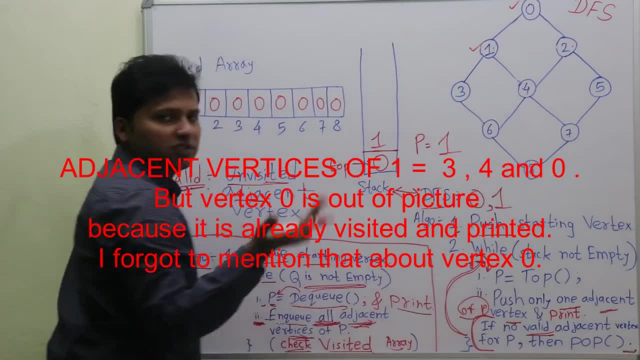 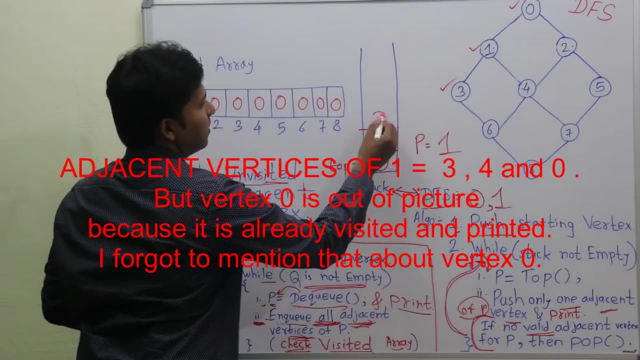 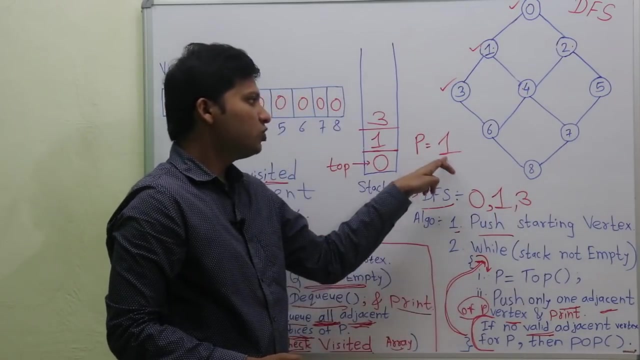 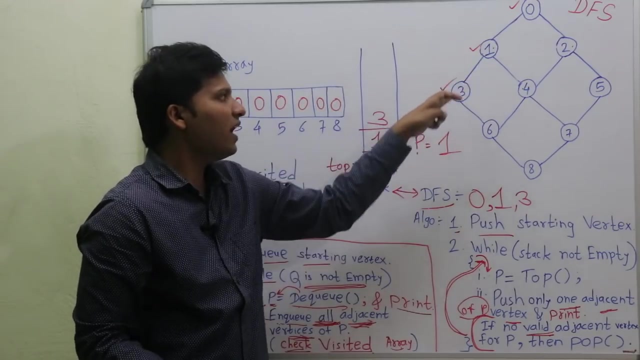 That is vertex 3 and vertex 4.. So proceed with any 1 vertex. So I proceed with vertex 3.. So I push this vertex in the stack and I print that vertex Right. So see. P points to 1. and this condition does not make a problem for P, because P has valid adjacent. 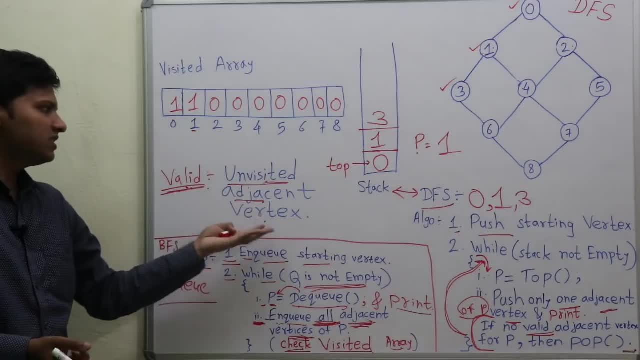 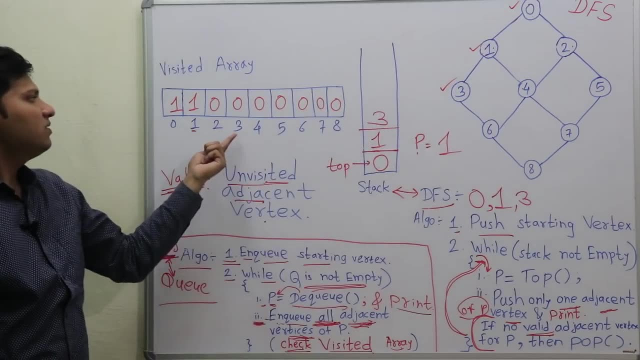 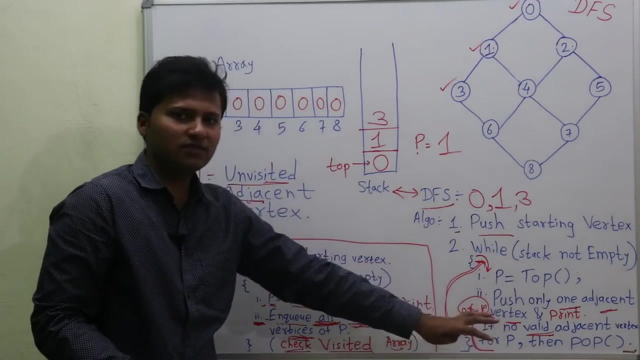 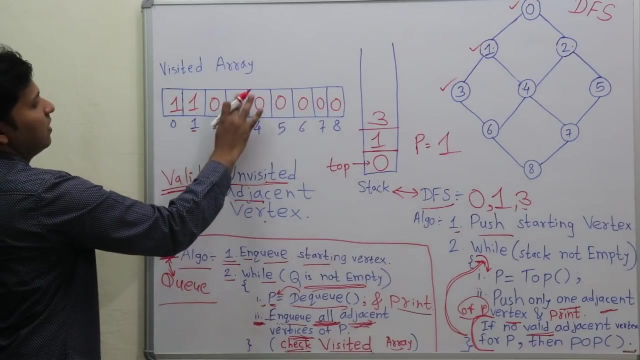 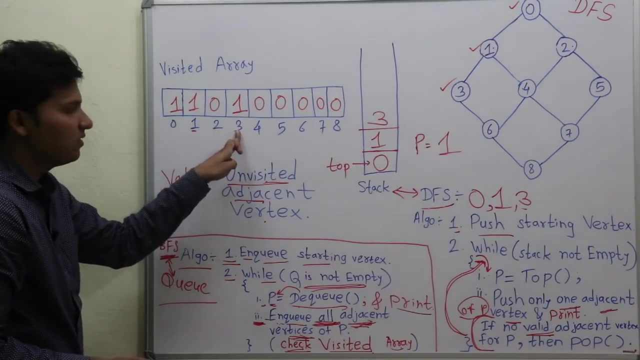 vertices now because P has unvisited adjacent vertices. See here for vertex 1. the vertex 3 is the adjacent vertex and vertex 3: it is yet unvisited, so it is a valid adjacent vertex. okay, so there is no problem for P. So as we have printed 3 and pushed 3, let us make the flag as 1, because now 3 is visited. 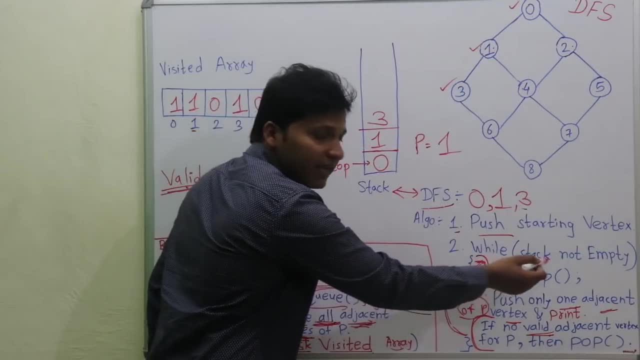 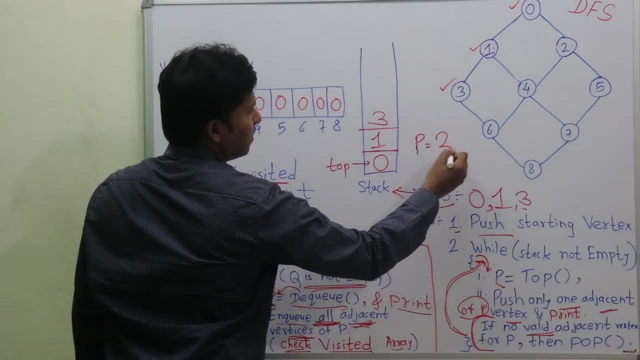 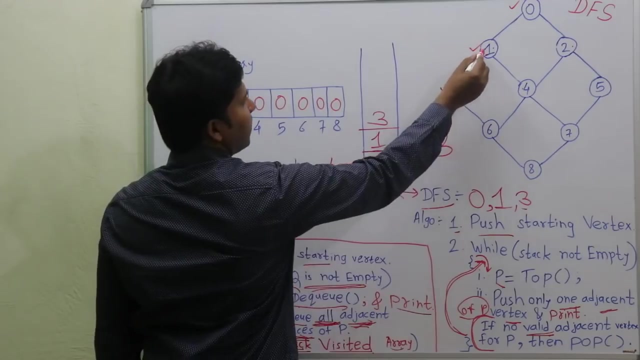 right, let us go to the next iteration. So while stack not empty, let us go inside. that is, P is equal to top, so what is the top element? that is 3.. So for 3, let us Check the adjacent vertex. So the adjacent vertices are vertex 1, vertex 6, but vertex 1 is already visited, right? it? 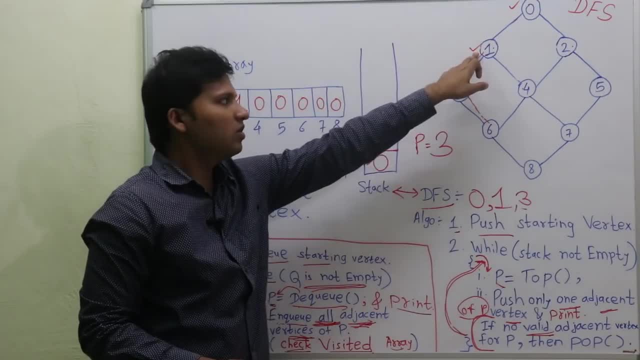 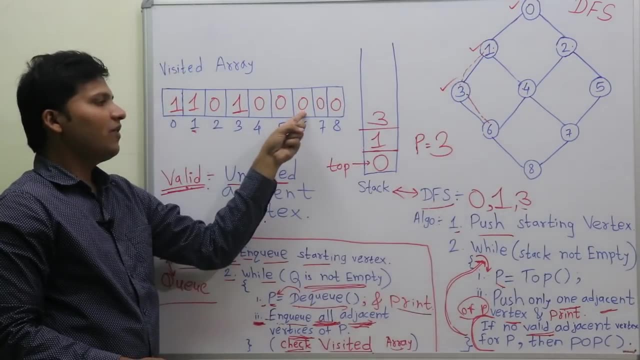 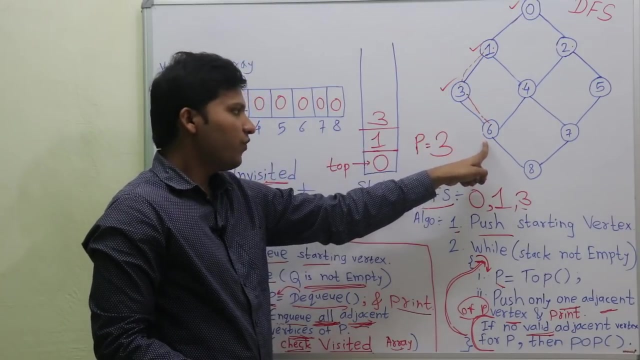 is already visited, so it is not in the picture now because it is not valid. so there is only one valid vertex, that is vertex 6. so check for vertex 6. the value is 0, so it is yet unvisited means there is valid, unvisited vertex here. 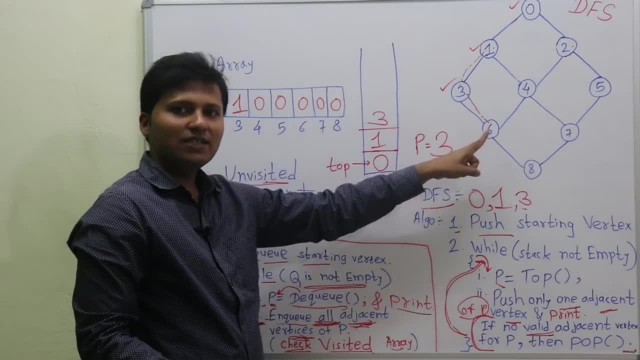 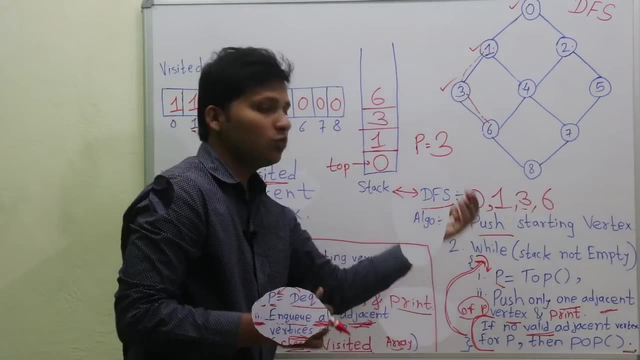 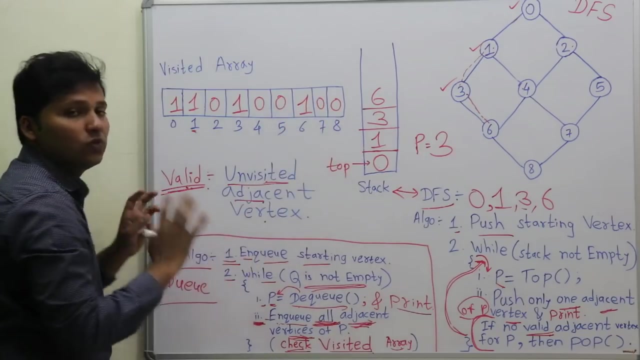 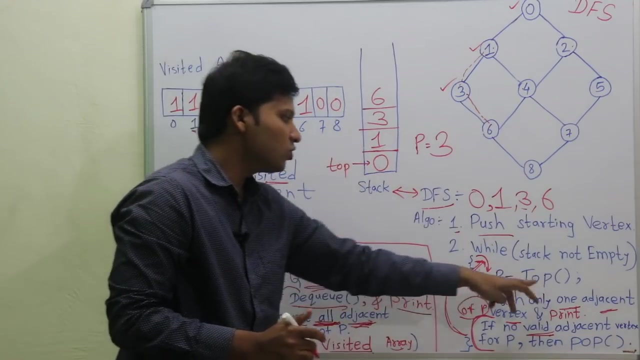 So for vertex P, The adjacent vertex is vertex 6, so push that vertex in the stack and print that vertex. So now, as 6 is printed, now you have to make the flag for 6 as 1 as it is visited. So let us go to the next while iteration. stack not empty. yes, the stack is not empty, so take. 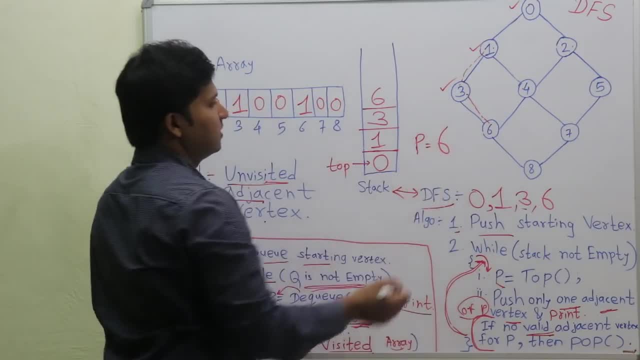 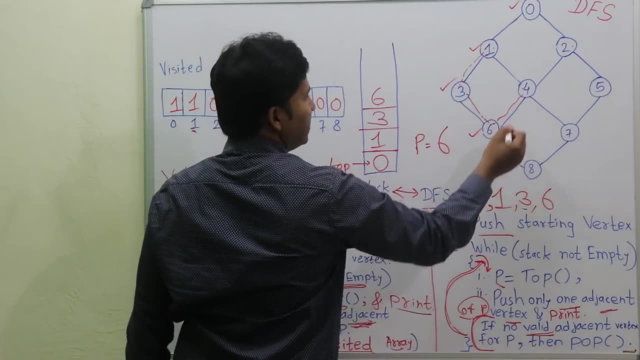 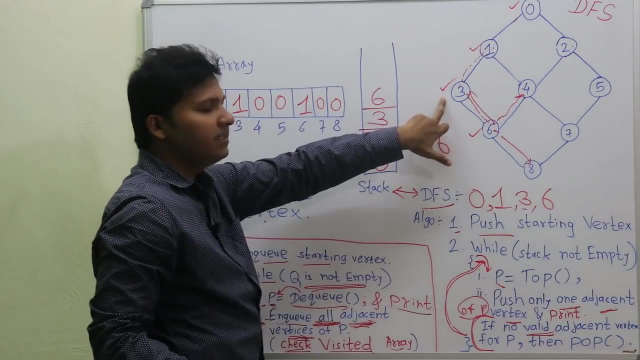 the top element. so top element of stack is 6.. Now for 6.. Check the adjacent vertex. so vertex 4 is adjacent, then vertex 8 is adjacent and vertex 3 is adjacent, but vertex 3 is not in picture because it is already visited. see, it is already visited. 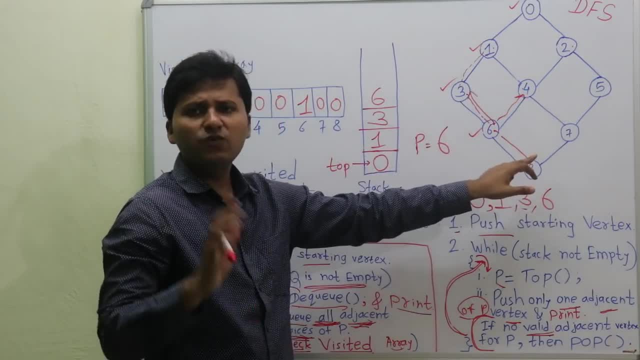 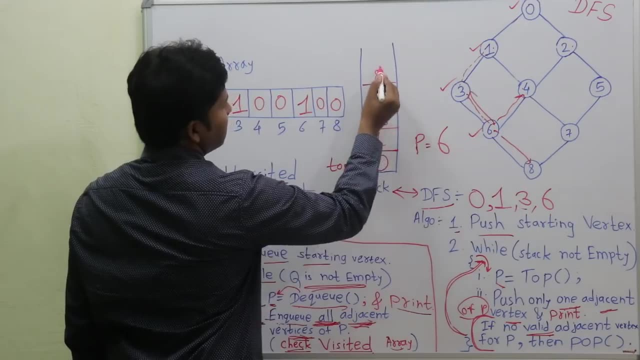 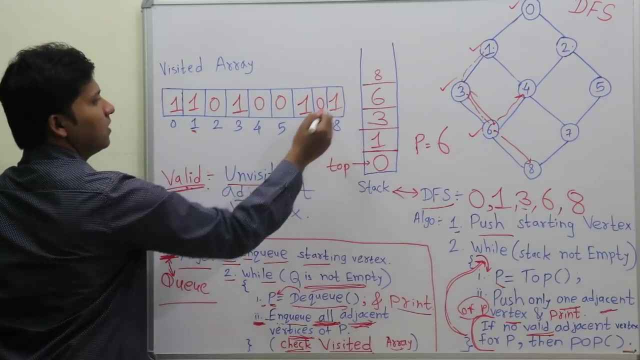 so out of vertex 4 and 8 you have to take any one vertex, so I proceed with vertex 8.. So let us push vertex 8 in the stack And Print vertex 8 and set the flag as 1. ok, now you remember the steps right, so again, go in the next while. 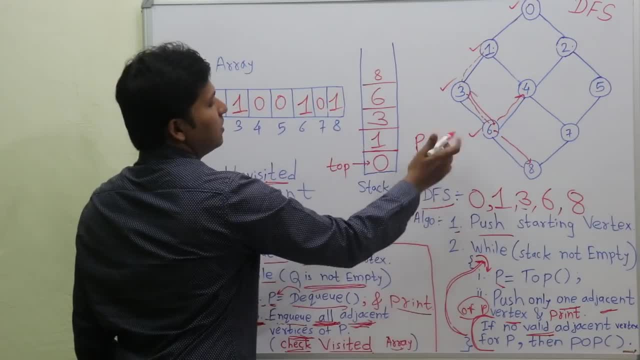 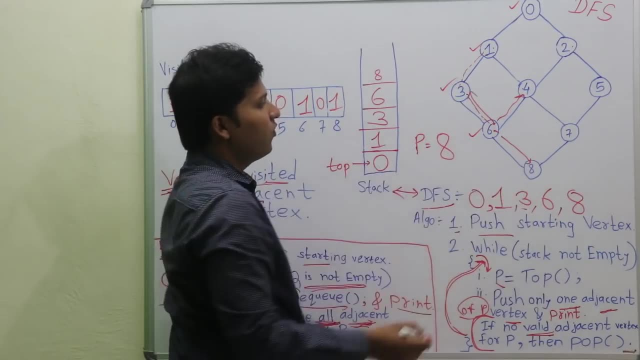 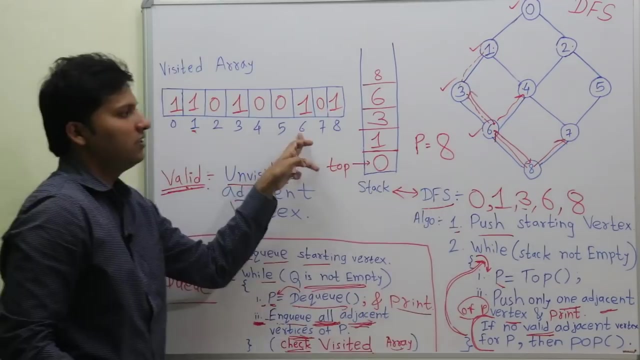 iteration. so P is equal to top. so 8 is assigned to P now. so for 8, check the adjacent vertices. see for 8. there are 2 adjacent vertices, 6 and 7. but 6 is not in picture because it is already visited. 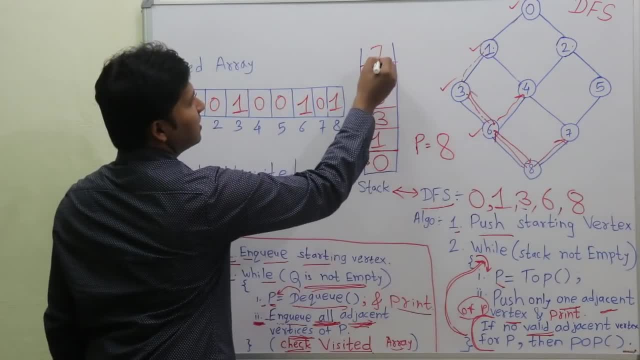 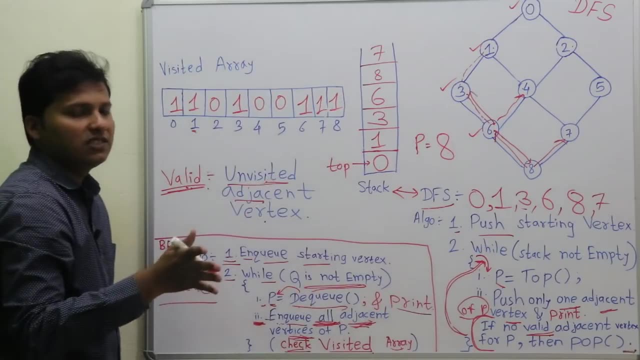 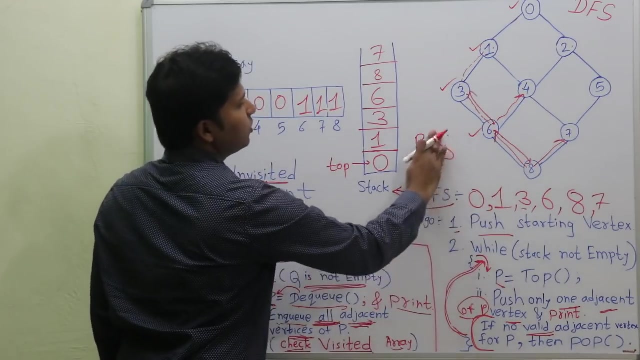 So 7 is the adjacent vertex. So push 7 in the stack, print 7 and make the value here as 1 because it is visited. so now let us go to the next iteration. so for vertex 7. so P is equal to top, so P points to 7 now. 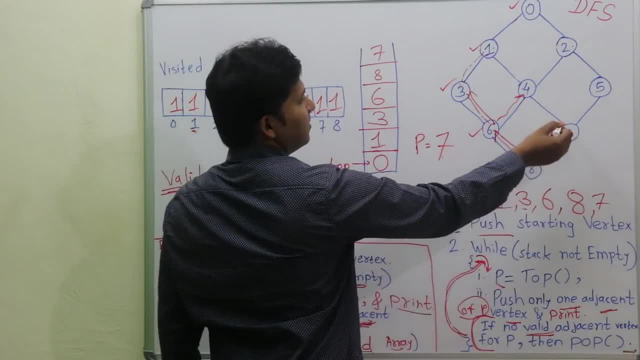 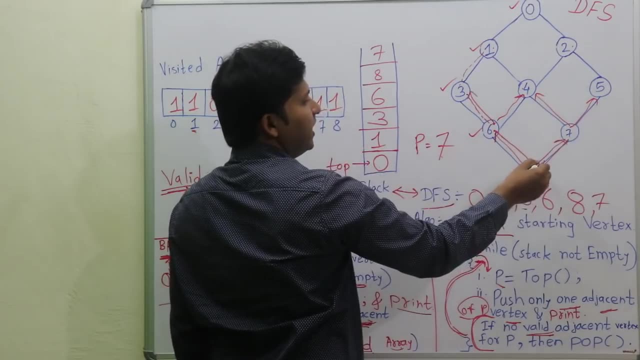 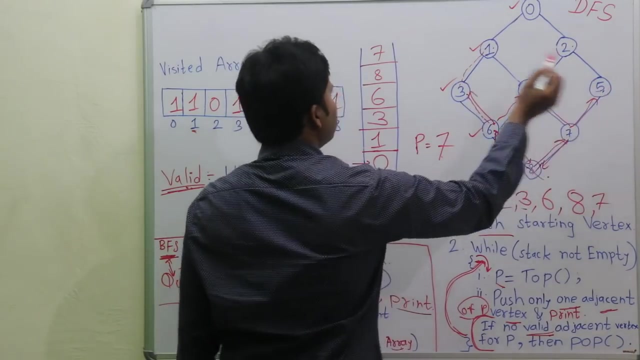 so for vertex 7, check for adjacent vertices: see. adjacent vertices are 4, 5 and 8. so out of 4, 5 and 8.. 8 is not in picture. So out of 4 and 5, we can proceed with 5. ok, so push 5 in the stack and 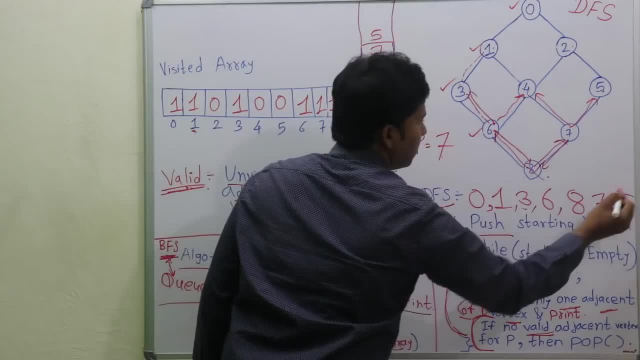 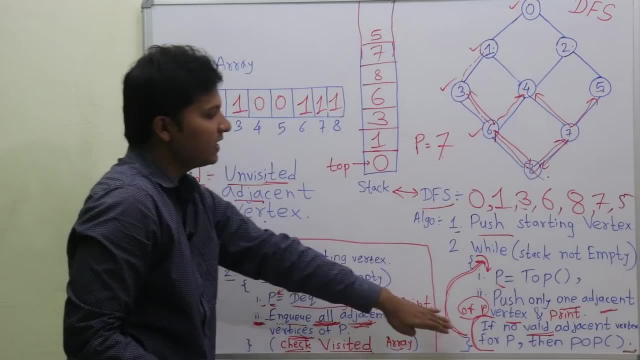 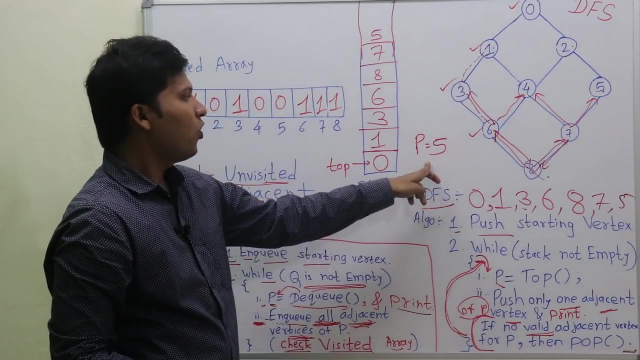 Print 5. ok, so I pushed 5 in the stack and printed 5. so again, let us go to the next iteration. so P is equal to top means P is equal to 5. ok, So 4, vertex 5.. So the next iteration is for the adjacent vertices, see 2- 7.. 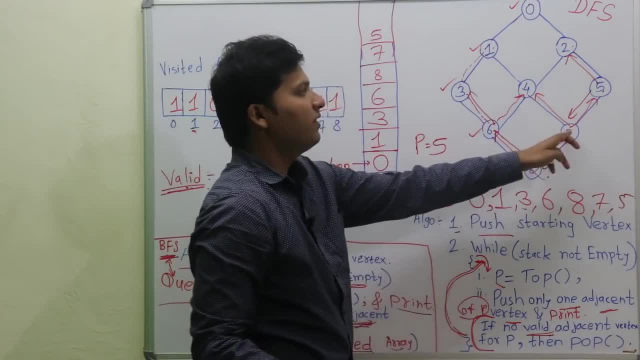 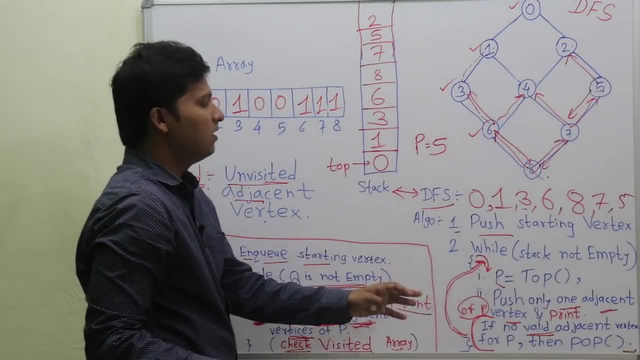 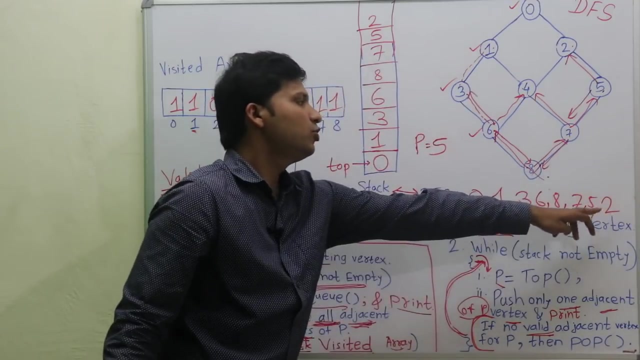 So 7 is not in picture, so we will proceed with 2. so now push 2 in the stack and print 2 here. I will just clean it. so print 2, ok. So I printed 2 here for the DFS traversal. So 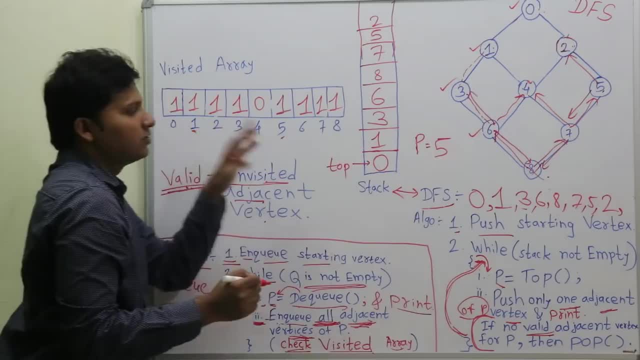 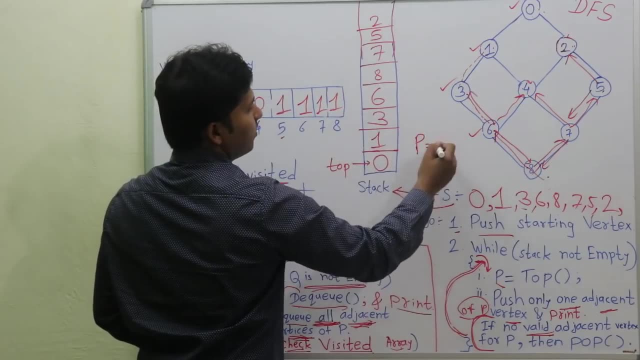 4, vertex 2.. So you make the flag as 1 for vertex 2 here. so now let us go to the next iteration here. so top. So now p becomes 2, p points to vertex 2.. So for vertex 2, check the adjacent vertices. 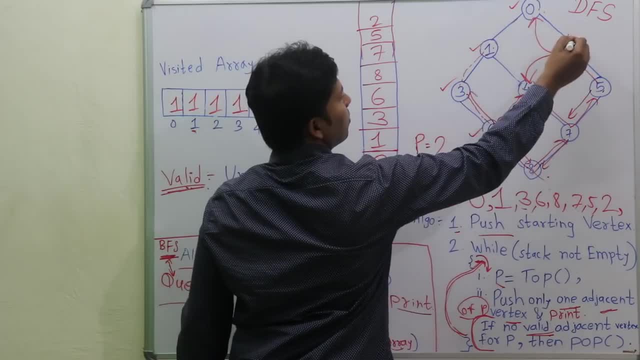 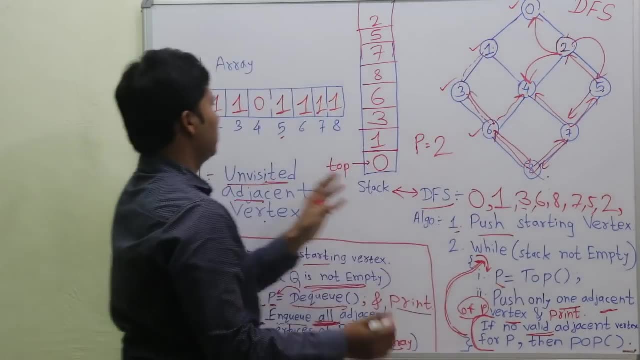 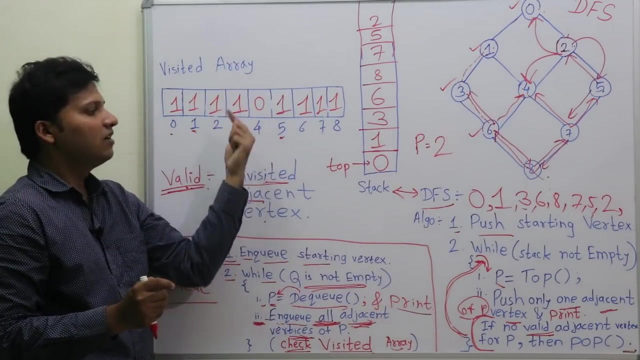 So see 4, then 0 and 5.. So out of these three vertices, see 0 and 5 are not in picture because 0 and 5 are already visited. So only vertex 4 is remaining. See 4 is unvisited. 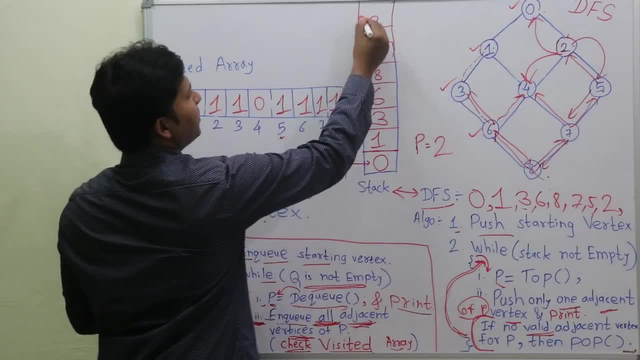 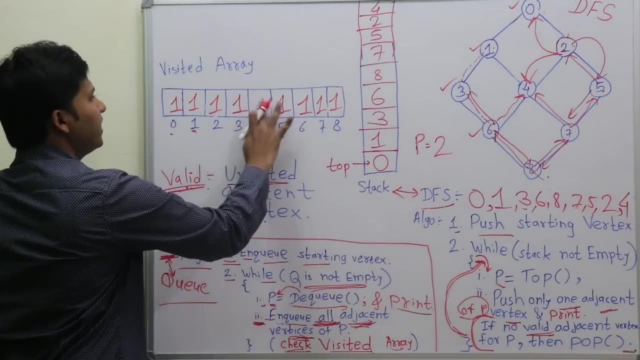 So that is the valid vertex. So push 4 and print 4.. So I print 4 here. So I pushed 4 and printed 4 and I make it 1 here in this visited array. So now let us go to the 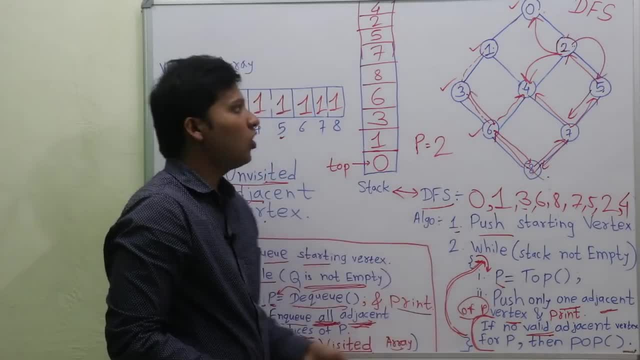 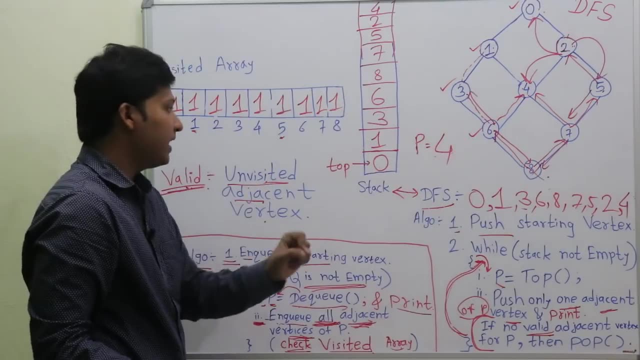 next iteration while stack not empty. Now see: p is equal to top, Now p becomes 4.. So is there any valid adjacent vertex for that? See what is valid Unvisited adjacent vertex. So that is the valid vertex. So now let us go to the next iteration. while stack not empty. 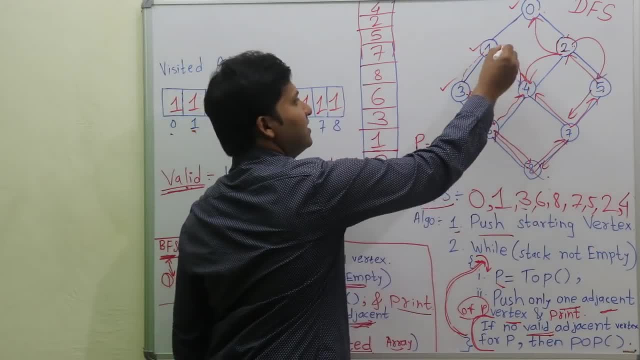 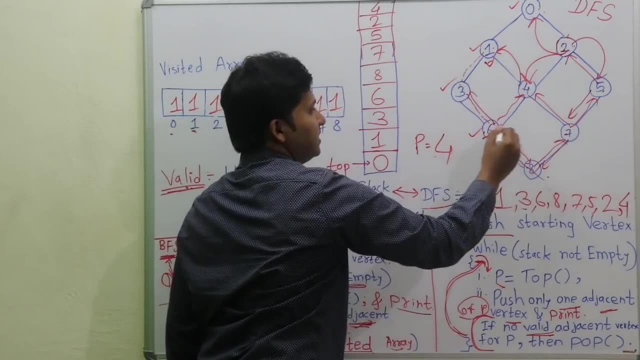 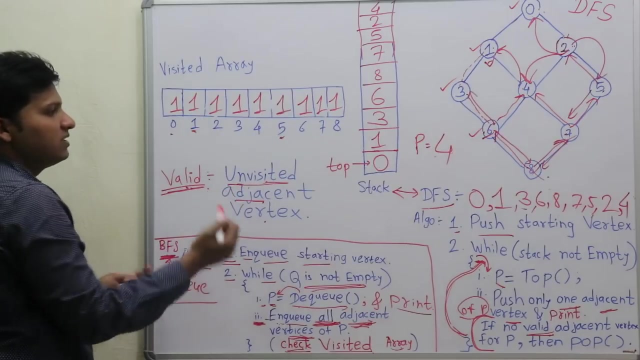 So for vertex 4, the adjacent vertices are 1,, 2,, 6 and 7.. So out of 1,, 2,, 6 and 7, nothing is valid, because all are visited. There is no unvisited vertex, So nothing is valid. So now you have to. 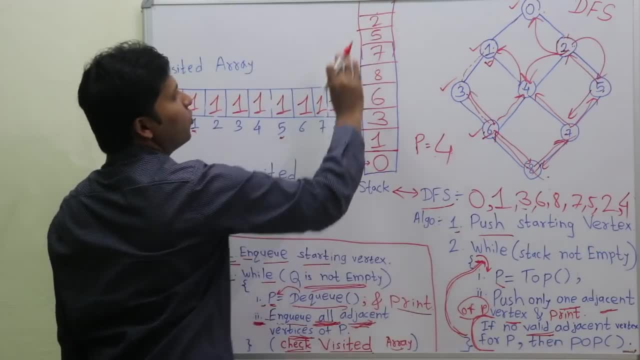 pop, So pop. element from the stack. So 4 is popped now. So let us go ahead to the next iteration. Still, there are a lot of vertices, So let us go ahead to the next iteration. So let us go ahead to the next iteration. So let us go ahead to the next iteration. So there are elements in the stack. 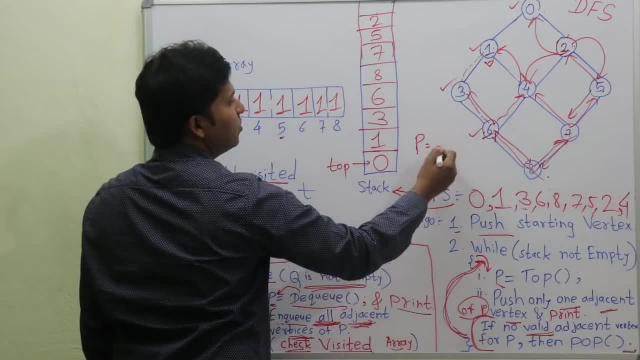 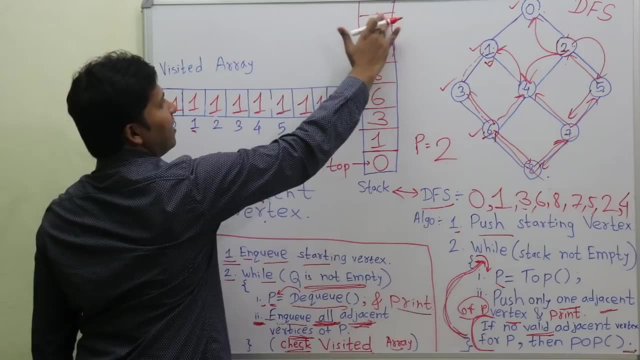 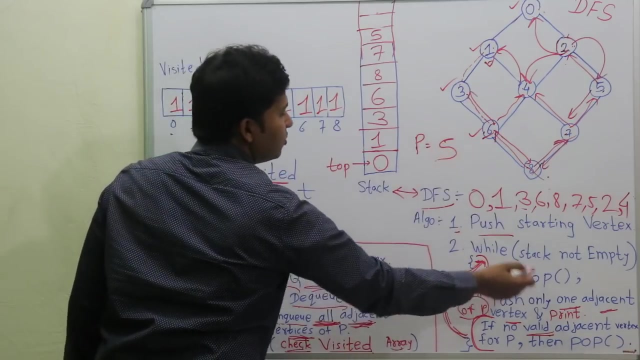 So p is equal to top. Now p is equal to top means p is equal to 2.. Again for vertex 2, there is no valid adjacent vertex, So you pop that element. So again go to the next iteration. Now p is equal to 5, because p is equal to top, So p is equal to 5.. Now vertex 5 also. 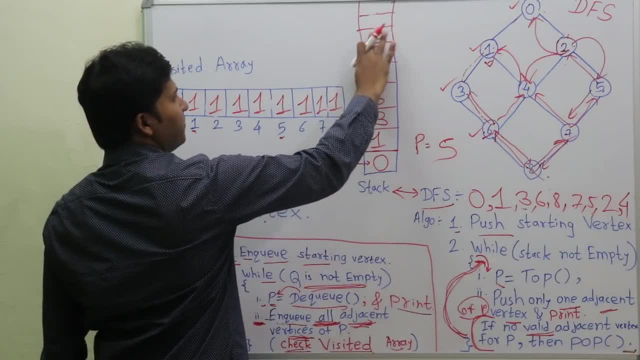 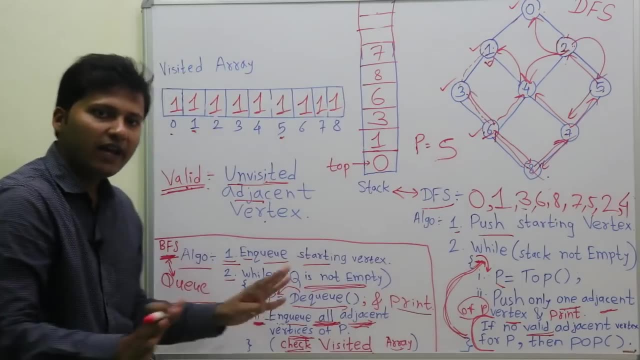 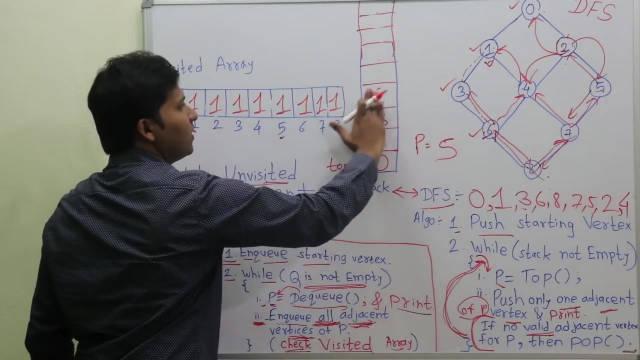 there is no valid adjacent vertex, So you pop 5.. So in this way, for any vertex in any iteration, there is no valid adjacent vertex Right, Because all vertices are visited. So all elements are popped one by one Right Now, when 0 is popped here. 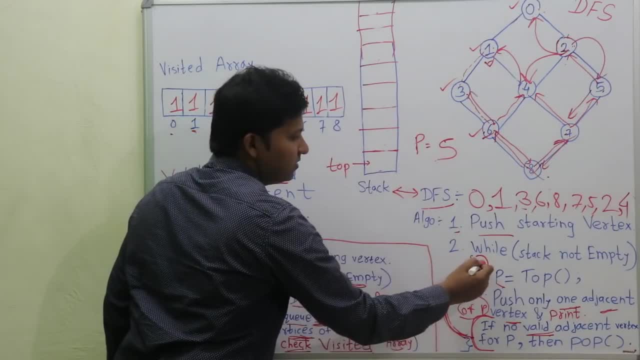 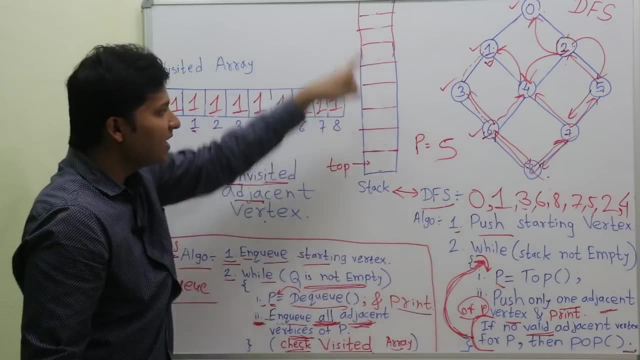 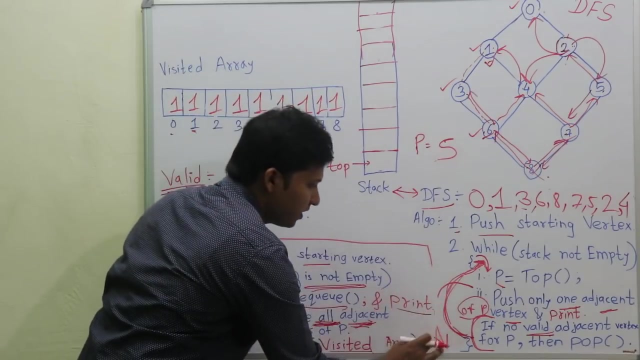 when 0 is popped. in the next iteration, after 0 is popped, we check while stack not empty. This condition fails because now stack is empty. out of this while loop, We come out of this while loop. So when we come out of this while loop, 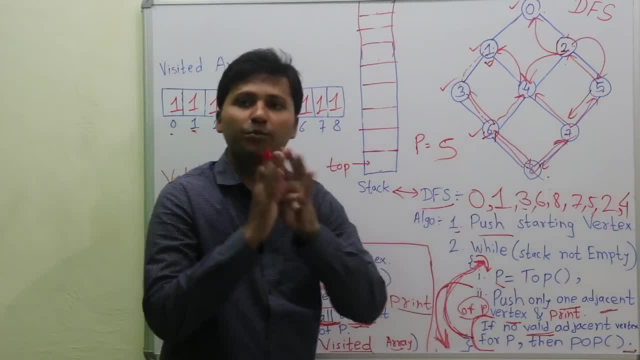 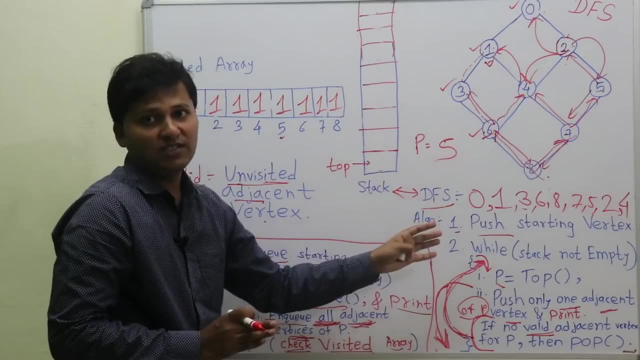 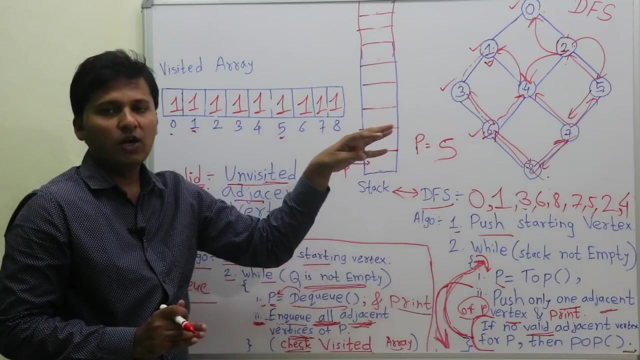 you come to know that the whole DFS is printed and our work is done. So in this way, using a stack, we print the DFS traversal. So in the next video we will see some more examples. See, this is a totally closed graph Now. in the next video we will see examples for some open graphs. So do watch.